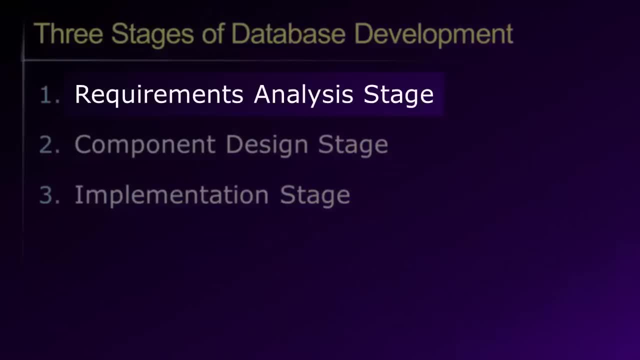 The first stage prior to actually developing a database itself is to perform what we call requirements analysis. This is the process of gathering information so that we can understand the data problem for which we are attempting to design a solution Once we have completed requirements gathering. 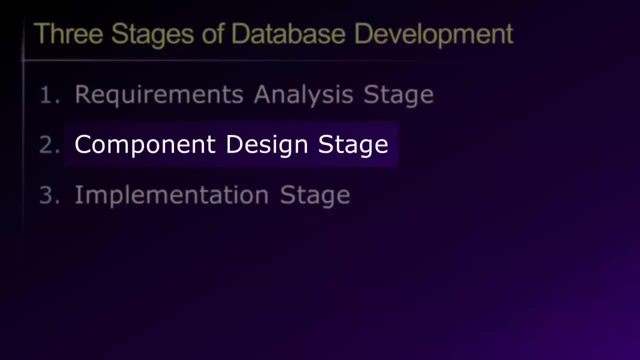 we can then move into the design phase, And the design phase is where we will create data models which are graphical. These are graphical representations of the database solution which we ultimately hope to implement. Finally, the third stage of database development is actually implementing our database designs. 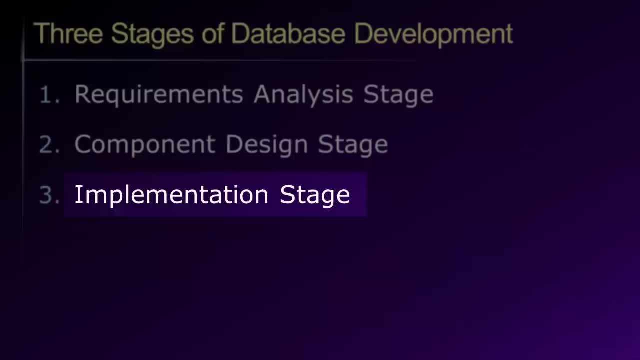 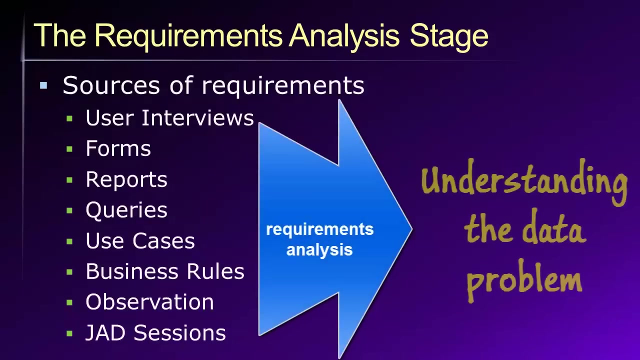 as a real world functioning physical database that can actually be used by an organization to solve one or more data problems. Broadly speaking, the requirements analysis stage is about gaining an understanding of the data problem for which we are trying to design a solution, And for this purpose we have many different possible sources. 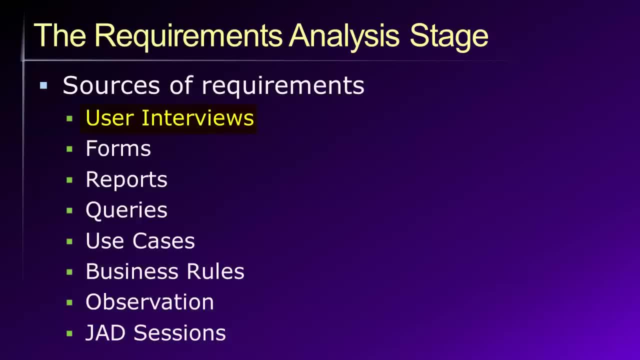 of information. They can include interviews with users, existing forms, reports or queries. So these might be forms, reports or queries that are used with a current system. If the organization is going through a broader systems design process, then use cases from within the unified 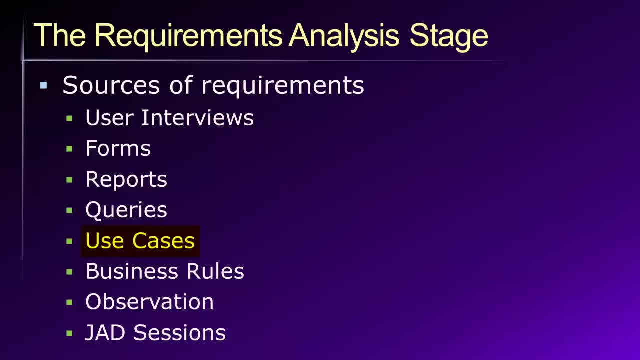 modeling language may be available to us. We may also consider business rules And observation, where we simply observe the way that various employees do their jobs in an effort to understand their data needs. And, of course, we may use JAD sessions. These are joint application development sessions. 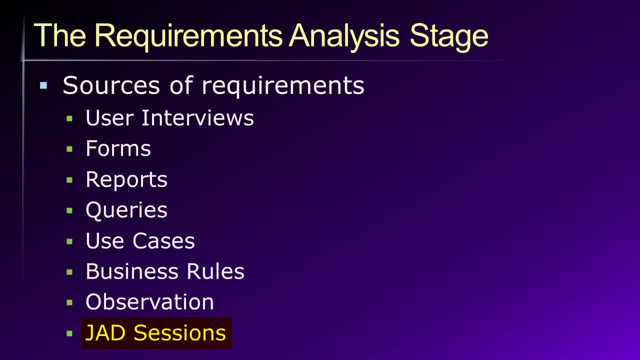 which are characterized by assembling all of the stakeholders in a project together in a single room. So you may have systems, designers, database designers, users, executives, potential customers, et cetera, And everyone in the room simply has a discussion about what they want the proposed new system to do. 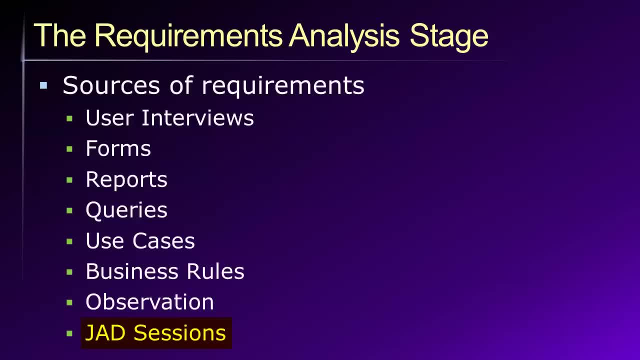 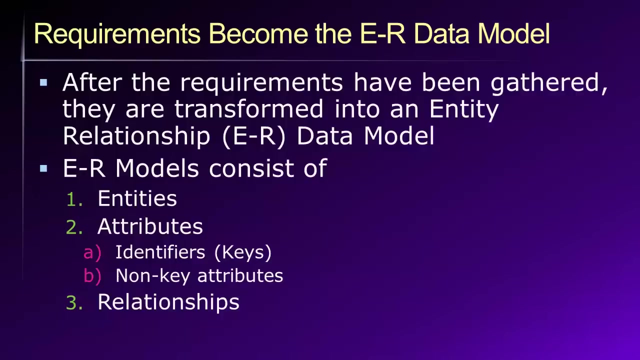 and how they want that system to function. Sort of information gathered from these joint application development sessions can then be very useful for developing a system in general and specifically, in our case, for developing the database to support that system. After we have completed requirements analysis: what we learn from that requirements? 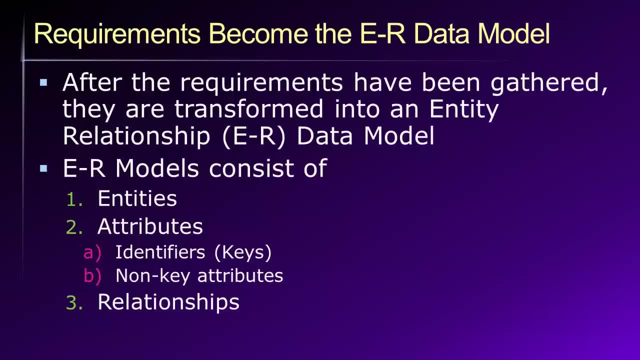 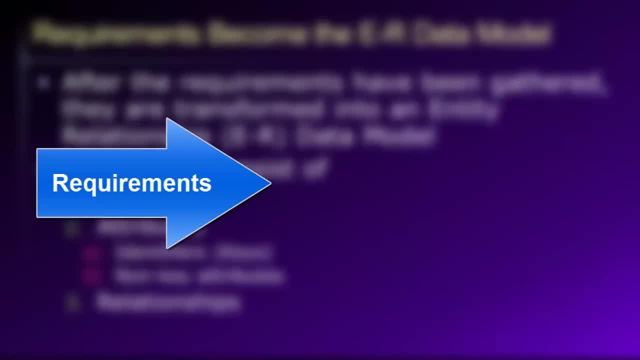 analysis process then becomes our data model. So we take everything that we learned through the requirements analysis stage and we process and distill all of that information into a data model, where a data model is a graphical representation of the database system that we ultimately hold. 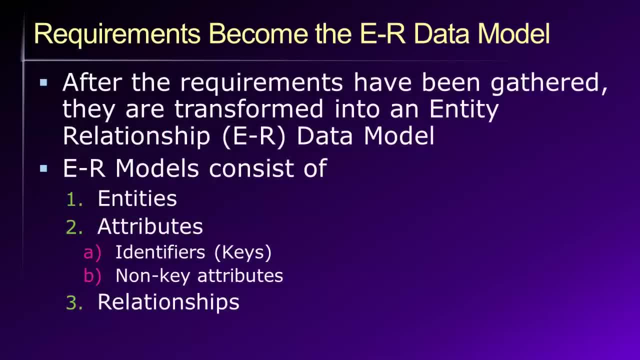 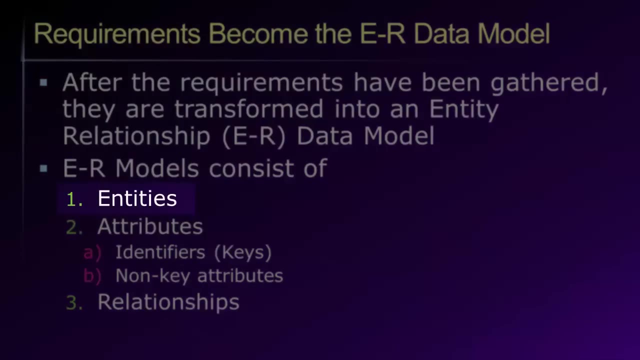 We hope to implement. The most popular type of data model that is used in the database world today is known as an entity relationship or ER data model. These ER models consist of three major graphical components. They are entities, which we have spoken about previously. 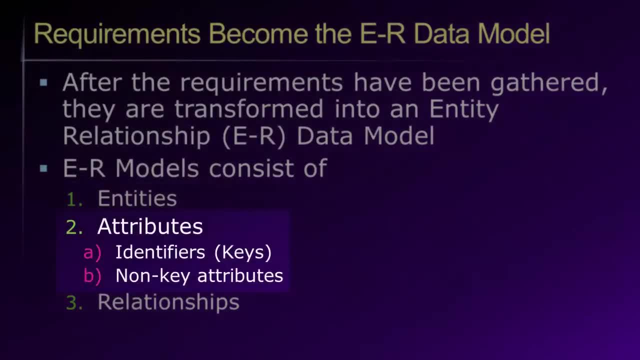 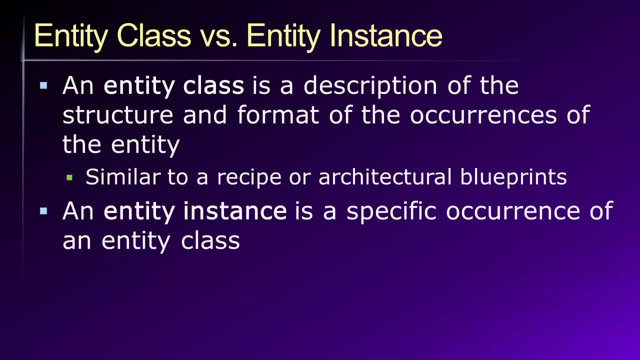 as tables or relations, attributes, for which several different types might exist, including identifiers or keys and non-key attributes. And our third and final component are relationships. These are relationships between entities. Before we proceed, I need to speak briefly about the distinction between an entity class and an entity. 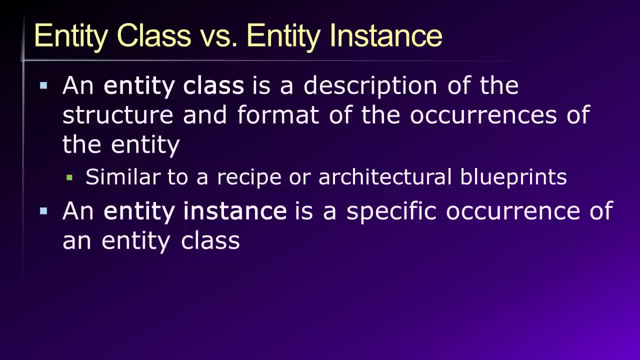 instance, An entity class Can be thought of as a structural description for the individual occurrences of an entity. I know that description contains a lot of technical jargon, So perhaps a better way of understanding this concept is to link it to other concepts which 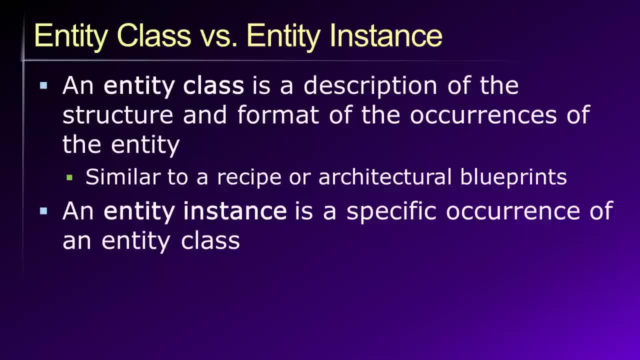 serve a similar purpose. Examples might be a recipe or blueprints that are used by an architect. In this case, let's consider a recipe for baking a cake. This is a generic recipe. we may have some basic instructions. we might do a simple, simple recipe with single ingredients. 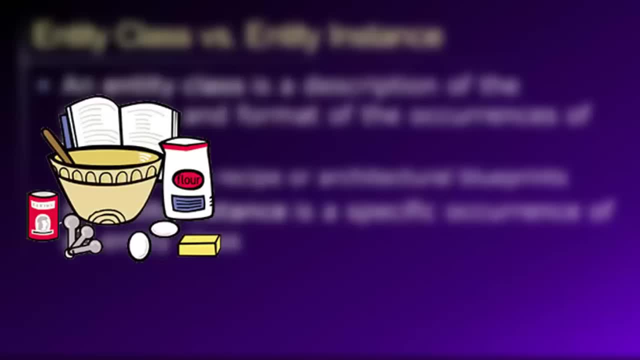 Mix powder 2-3, or powder 1-2-12,, flour 5-5, or המ-2höいく-3,, sugar 2½-3, or powder 2-3, or baking powder 2½-3, or. 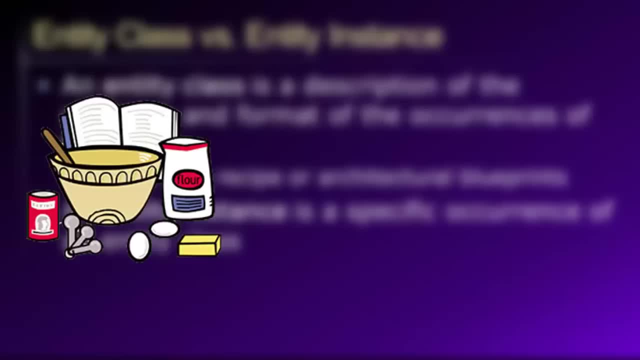 mix above ground extra flour 3-4, or mix the flour together with sugar and baking powder, put that in an oven, bake the cake and then we add an overall конечно value. the meant amount of became a positive. we add whatever sort of frosting we like. 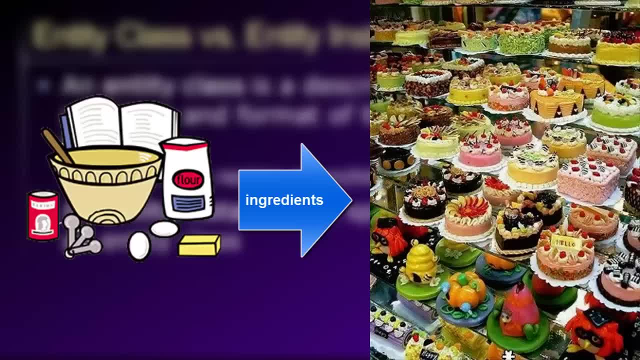 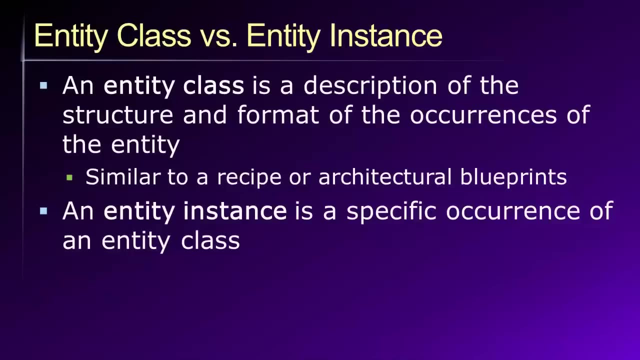 So the recipe gives us a basic framework or guideline on how to produce a cake, But ultimately the cake that is created is a unique, individual item. In our analogy, the recipe is equivalent to an entity class, while the resulting specific, individual real world cake. 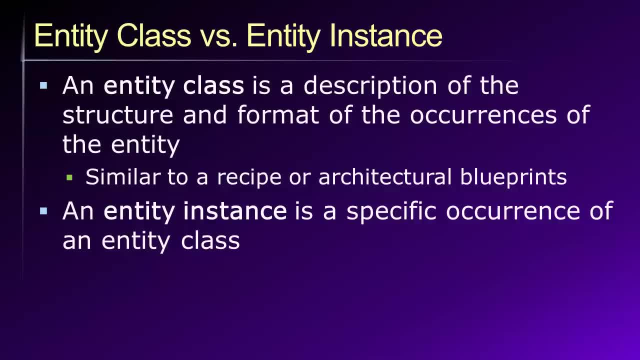 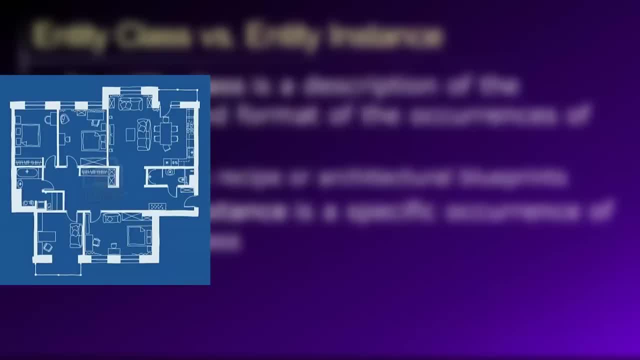 is equivalent to an instance of the entity. Similarly, we might consider architectural blueprints, where we may have a generic set of blueprints that tell us how to design a basic house, But then the homeowner, who is building the house, may be able to make some specific decisions. 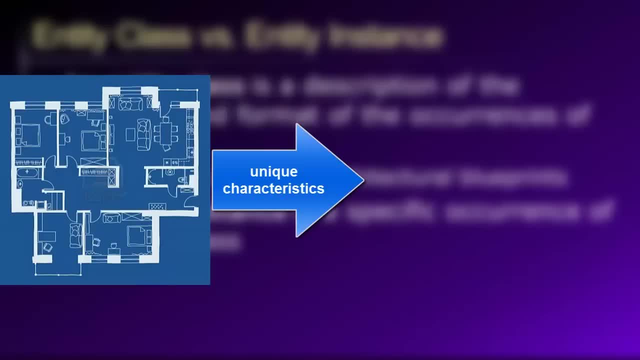 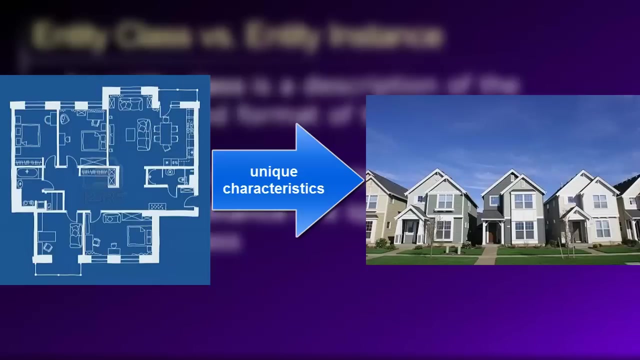 such as what type of appliances they want to use And the kitchen, or what color they want the paint to be, or what type of carpeting they want. All of those individual characteristics make the resulting real world house a unique, specific item. 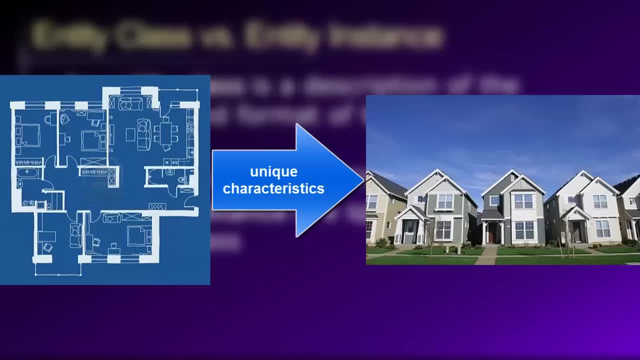 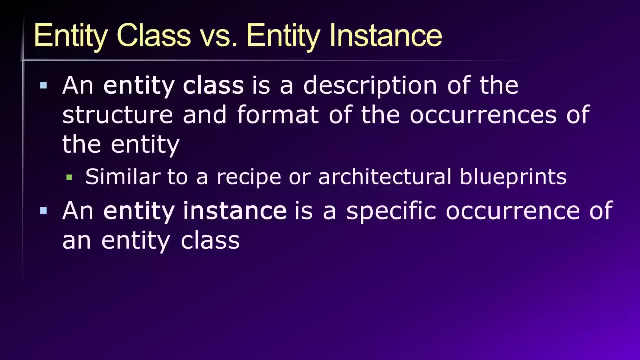 In our analogy, the architectural blueprints are similar to an entity class, while the resulting individual real world houses that are created as the result of following those blueprints would be instances of the entity class. So just remember that an entity instance is an occurrence of an entity class. 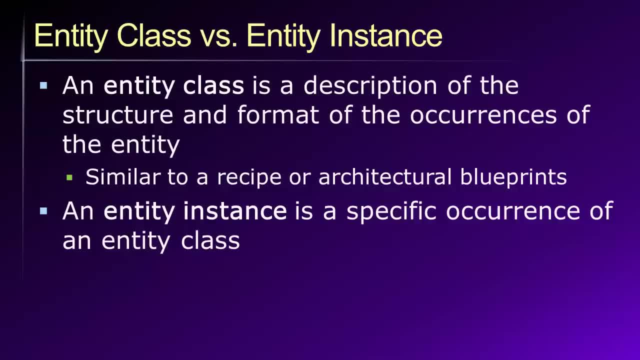 If we have an employee entity, that is, an employee entity class, we may define attributes that we want to track for all employees, such as an employee entity number, an employee ID number, an employee name, an employee department, When we add a new row of data to that table. 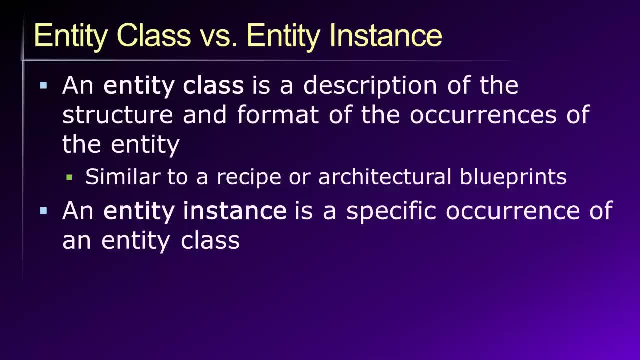 and we specify specific values for those attributes. perhaps employee ID number one named Dan who works in the marketing department. we are describing a real world entity. that new row of data is an instance of an employee And, as far as the database is concerned, 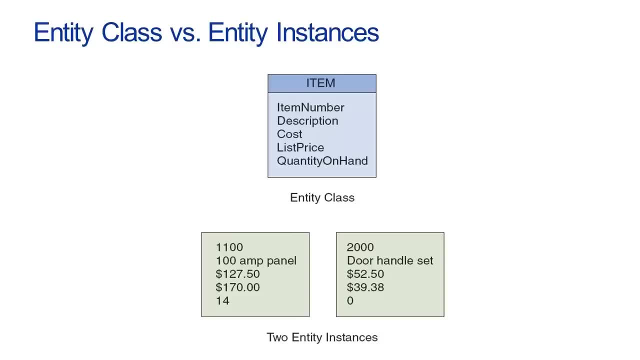 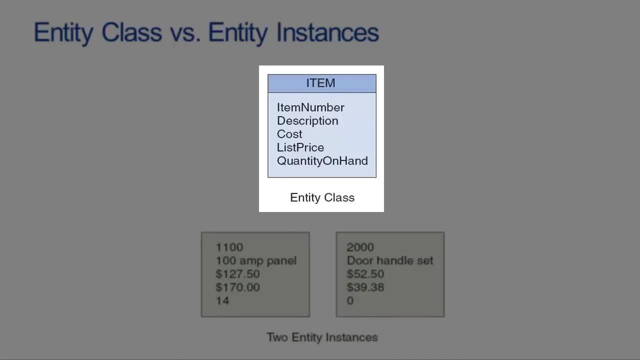 that row of data is an employee. Here we see some additional examples. Our entity class in this case is an item, And we can see that the item entity contains five attributes: item number, description, cost, list, price and quantity. 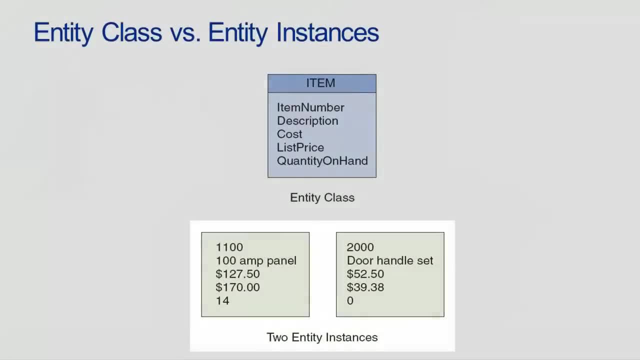 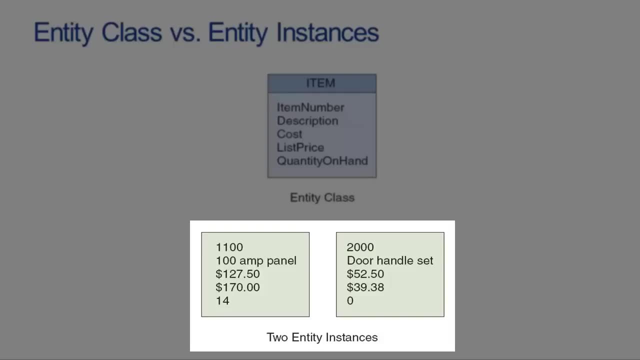 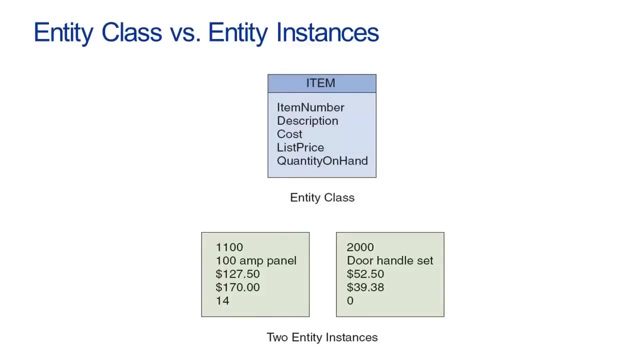 on hand And then we see two Instances of that entity. So the instances of the entity represent an instantiation of the entity class. This idea, if you've had some object-oriented programming, is directly analogous to the concepts of a class and an object in the object-oriented programming. 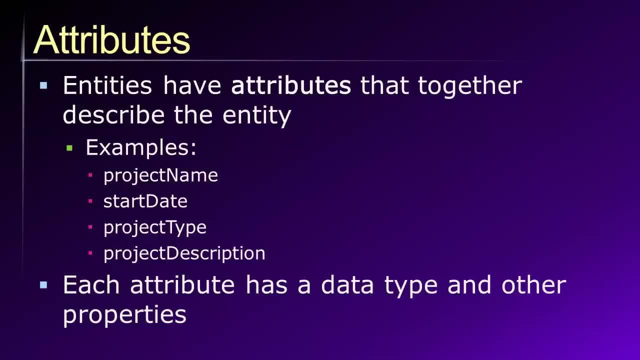 paradigm. Next, I would like to talk about attributes. An attribute is a specific piece of information that we would like to keep track of for each instance of an entity. If we're talking about an employee, we may have attributes that we want to track, such as the employee's name or their age. 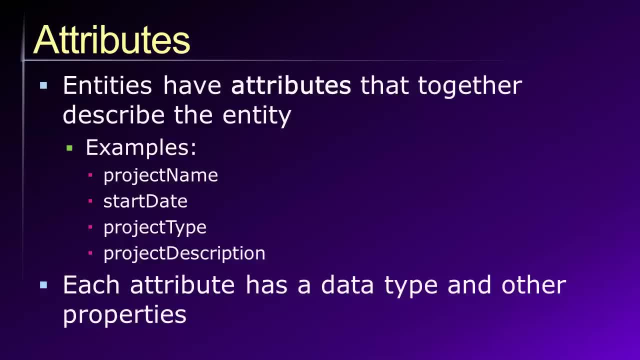 or the date when they were hired, and so forth. If we're talking about a project entity, we're talking about a project entity. If we're talking about a project entity, we're talking about a project entity. We may have attributes that we want to track, such as a project name. 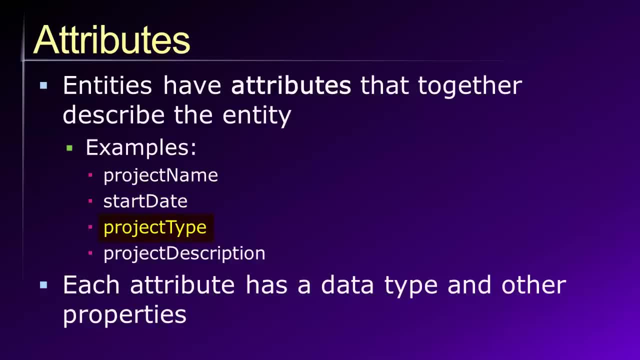 or the start date of the project, or the type of project, or a description of the project. The point here is that, as we fill in values for these individual attributes, what we are really doing is defining a specific instance of the entity class. 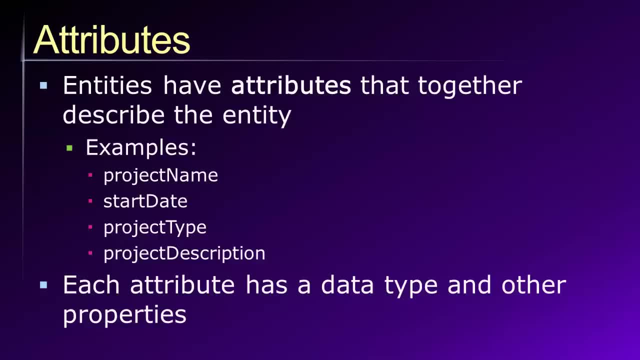 So we are defining an employee, Or we are defining a real-world project by providing values for these attributes. Each attribute that is part of an entity has a data type as well as several other properties, So we may define an employee ID number, for example. 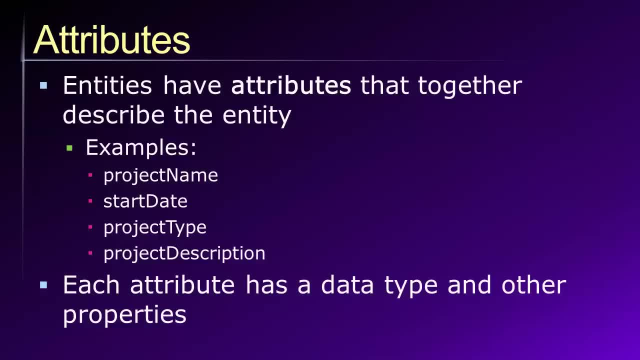 as an integer. We may define the employee's name as a VARCHAR with a maximum length of 50 characters. We can also specify additional properties for each attribute, such as whether or not the attribute is allowed to store null values, Or perhaps we want to provide a textual description. 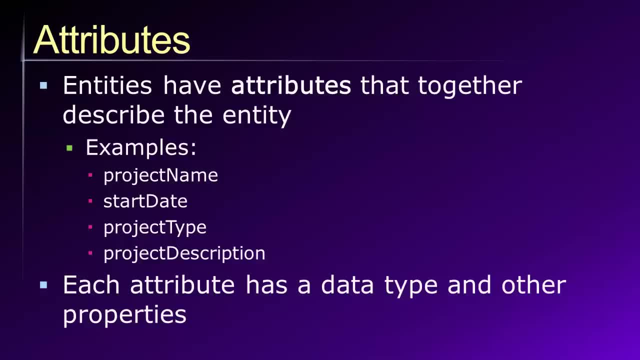 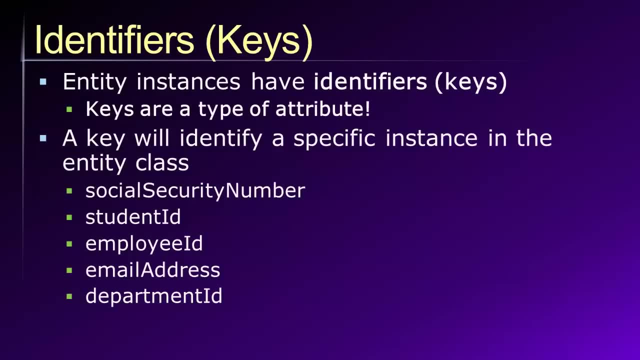 of the attribute. So, in addition to a data type, an attribute can have other properties as well. Broadly speaking, we can consider two different types of attributes. There are first identifiers, which we will generally refer to as keys, And then we have non-key attributes. 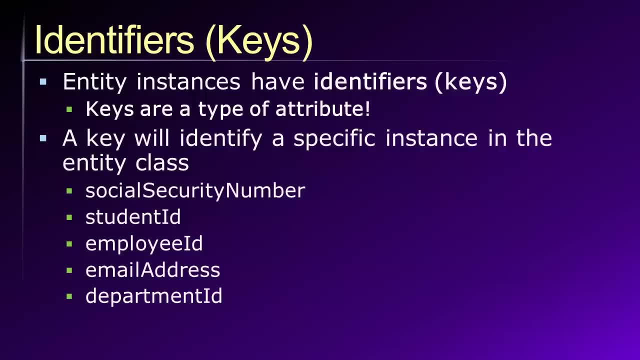 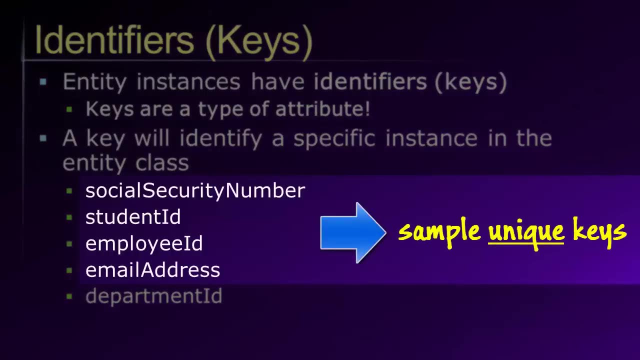 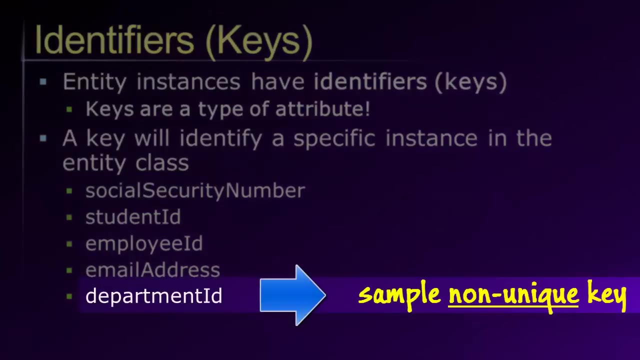 In the first case, identifiers are attributes whose values are used to identify an instance of the entity class. Common examples of identifiers or keys might be a social security number, a student ID, an employee ID, an email address or even a department ID. 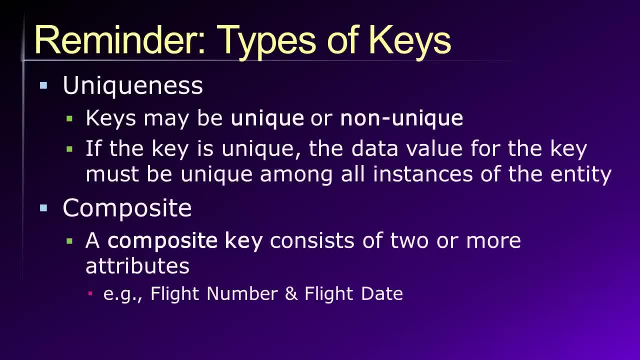 One of the important things to remember about keys is that they can either be unique or non-unique. If a key is unique, that means that each instance of the entity, or, if you prefer to think about it as each of the entities, each row in the table, will have a unique value. 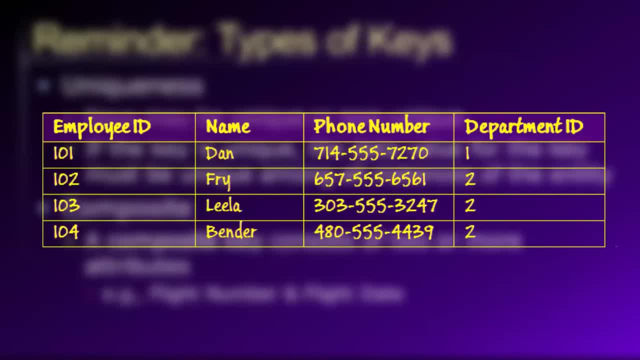 for that attribute. For example, our employees may have an employee number and we would almost certainly want each employee to have a unique employee number so that we can keep track of our employees individually by using that number. By contrast, we can also have non-unique keys. 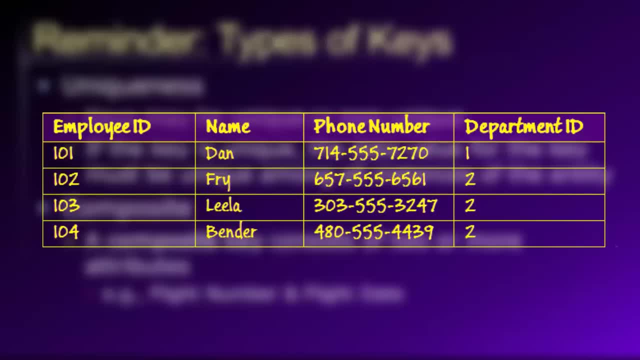 And non-unique keys are used in order to group instances of an entity class into categories. An example might be a department ID. More than one employee can have the same department ID, And what that tells us is that the employees which share the same department ID all belong to or work in. 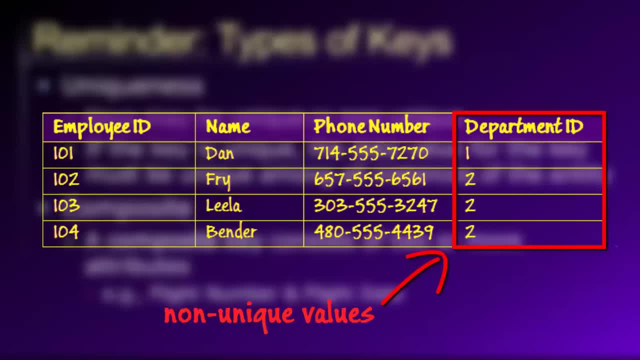 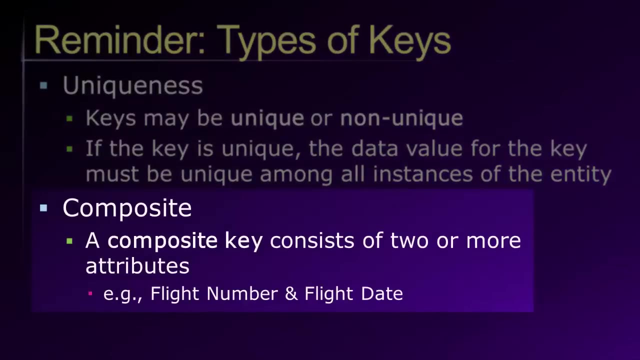 or are affiliated with the same department. In that case, the key would be non-unique because more than one instance of the employee class can have the same department ID. Recall also that we have composite keys and that a composite key gains its uniqueness by combining the values of two or more attributes together. 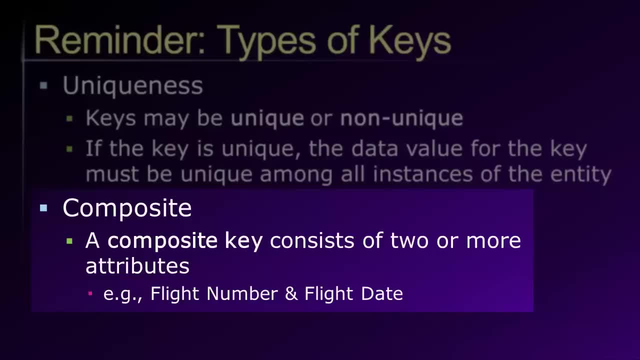 The example that we used previously in this series of lectures was the flight number and the date of a flight, So we may have, for example, United Airlines Flight 33 that takes place on the 17th of March 2016.. There may be several other flights that take place. 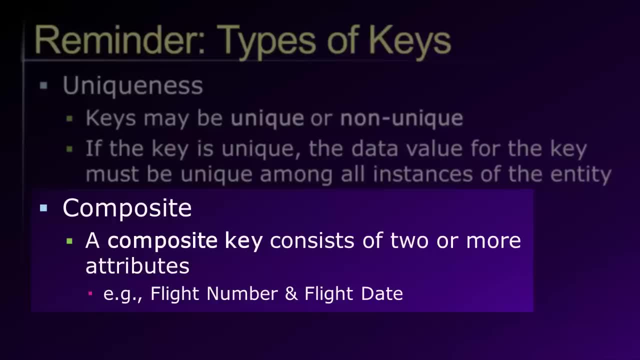 on the 17th of March And we may operate Flight 33 every day. But if we combine those values together, we can then use Flight 33 on the 17th of March to identify a specific real-world flight with a real airplane, real passengers and so forth. 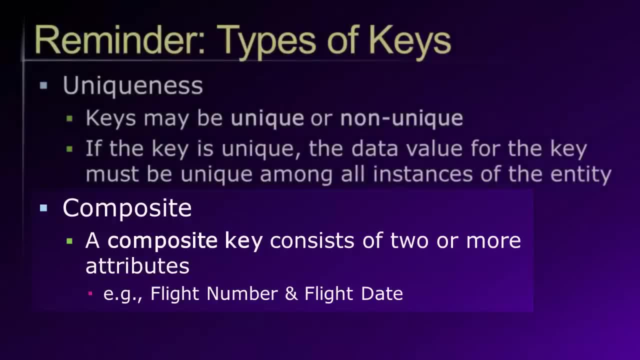 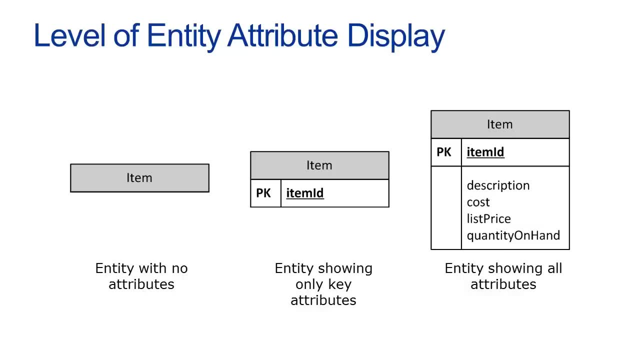 The combination of those two values will be unique. Before we continue our exploration of entity relationship models, I think at this point it would be a good idea to provide examples of different ways in which entities might be represented in an entity relationship diagram. The simplest way of representing an entity. 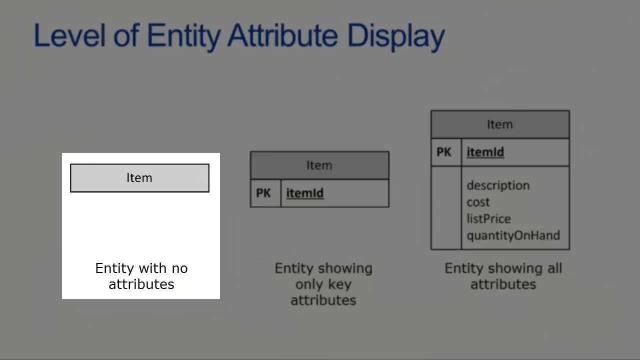 is just to use a rectangle which contains the name of the entity. This is usually used for conceptual data modeling. I may, for example, have an item entity. All I need to know is that an item entity is related to other entities in some way. 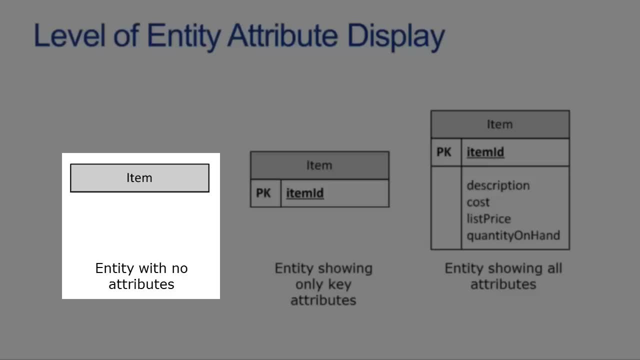 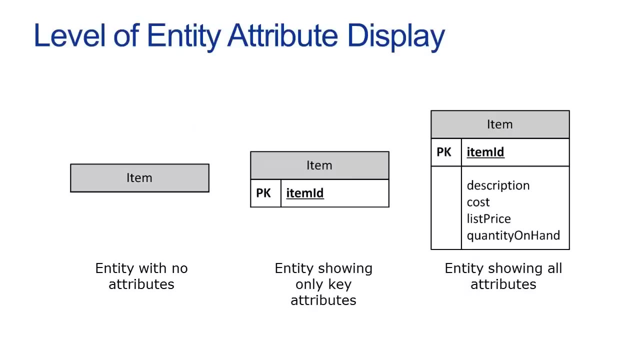 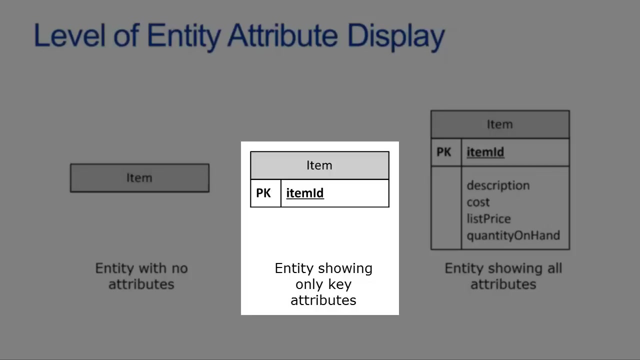 I don't yet care about the various attributes that will become a part of the item entity. Another way of graphically depicting these entities is to show the entity And just include its key attributes, attributes which are serving as identifiers or keys for the entity. 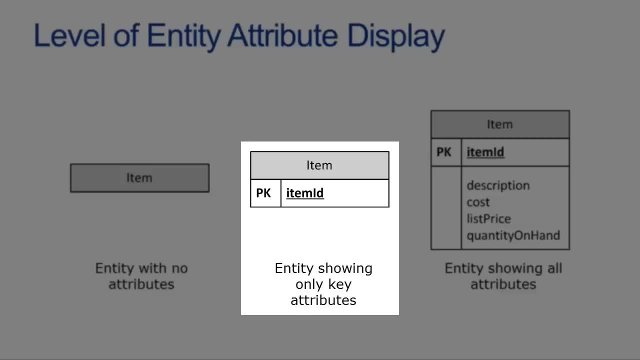 We might, for example, have an item entity And we may have defined an item ID as its primary key, And we will list just that single key attribute so that when we create relationships between the item entity and other entities, we can see which attributes are involved in the relationship. 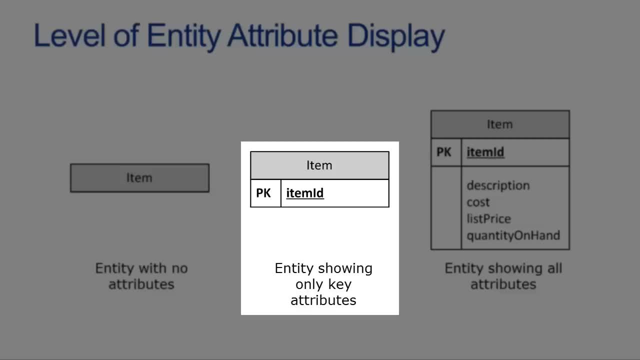 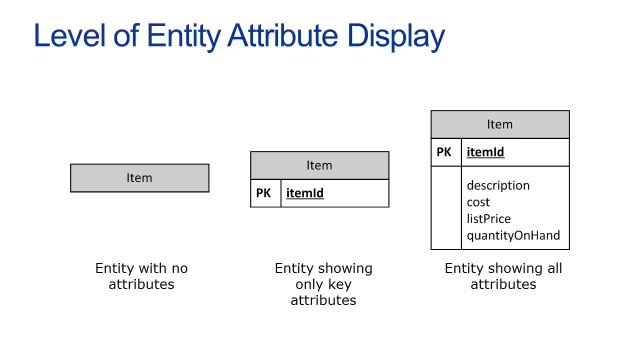 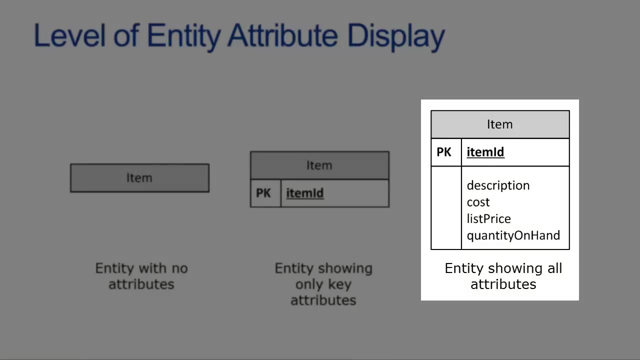 And that may be all of the information we need during a preliminary stage of data modeling. Finally, we have a way of representing an entity in its entirety, which includes not only the name of the entity and its key attributes, but also all of the other non-key attributes that together comprise 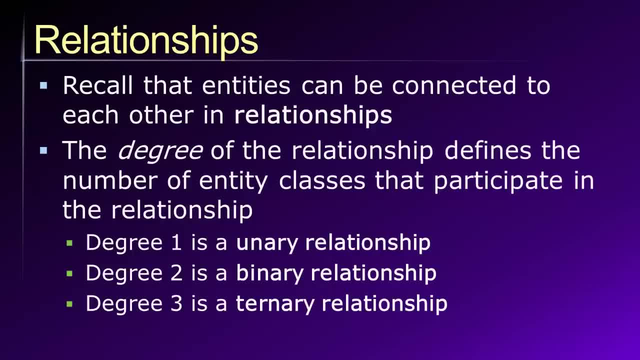 Next, I would like to talk about relationships between entities. If you recall from some of our earlier lectures, we talked about how relationships naturally emerge among the various business concepts for which we might want to track or record information. A department, for example, can have 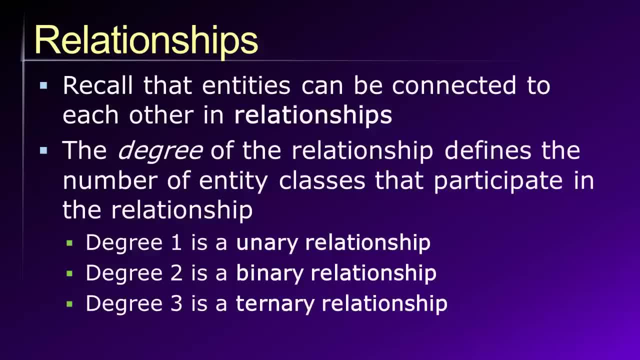 many different employees, Or a customer can place many different orders, Or a product can have many different suppliers. These are all examples of relationships among entities, relationships among business concepts. From the perspective of entity relationship modeling, then we can consider several different types. 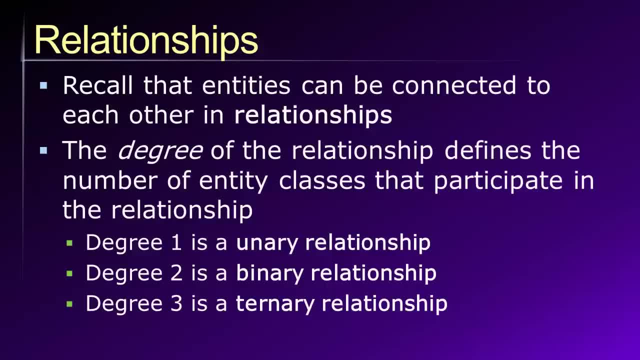 of relationships, And these types of relationships can be defined by what we call the degree of the relationship, where the degree of the relationship refers to the number of entities that are participating in the relationship. Common examples include a unary relationship. This would be a degree one relationship in which an entity 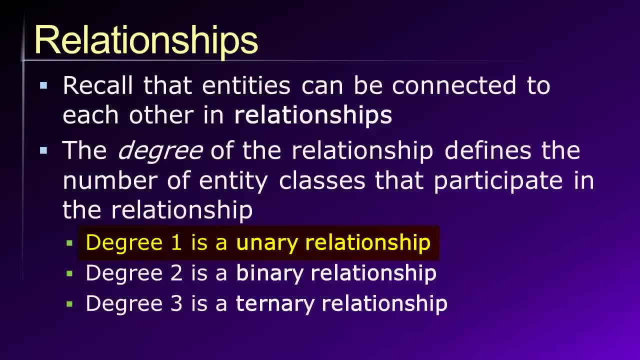 is related to itself. We would also call that a recursive relationship. We may also have a binary relationship or a degree two relationship, where one entity is related to another entity. Binary relationships are by far the most common types of relationships in entity relationship modeling. 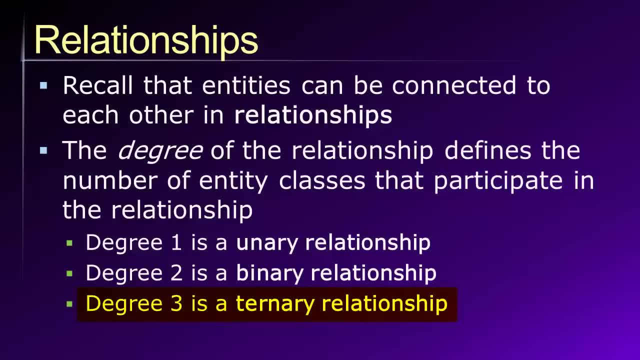 We may also have a ternary relationship or a degree three relationship. In a ternary relationship we would have three entities involved in the relationship, So the degree then simply refers to the number of entities which participate in the relationship. Let's see some examples. 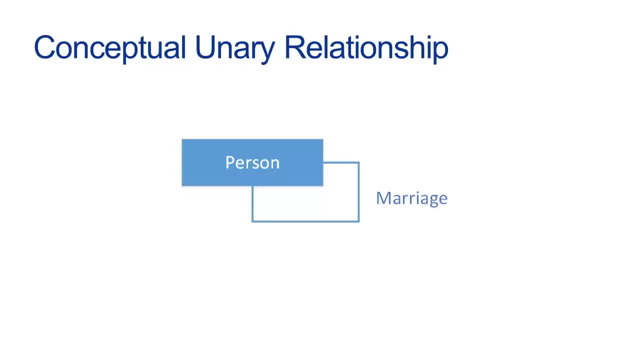 Here we see a conceptual drawing of a unary relationship. Remember that a unary relationship is an entity that is related to itself. In this case, we have a person entity and the person entity has a relationship to itself that we are calling marriage. What we can infer from this diagram, then? 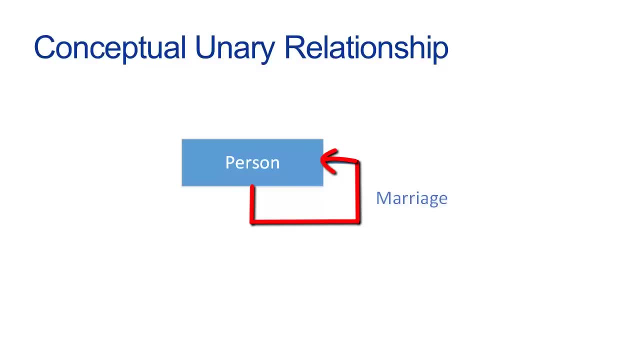 is that a person can be married to another person. The possibility exists for instances of the person entity to have this marriage relationship with each other. So a person can be married to another person. The person entity is related to itself in a unary relationship. 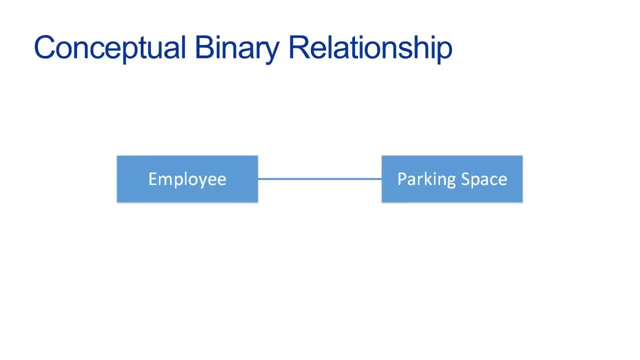 Here we see an example of a binary relationship. In this case we have two entities- employee and parking space- and these two entities are related to each other. So an employee may park in a parking space or a parking space may be assigned to an employee. 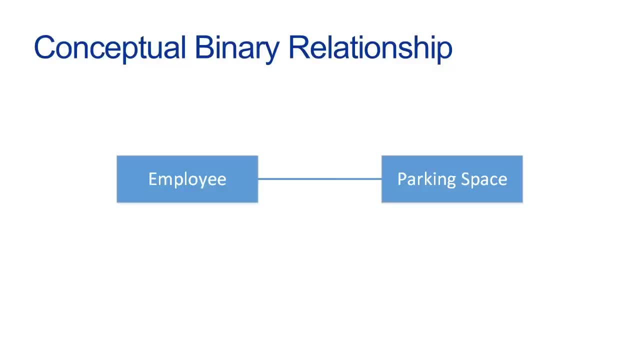 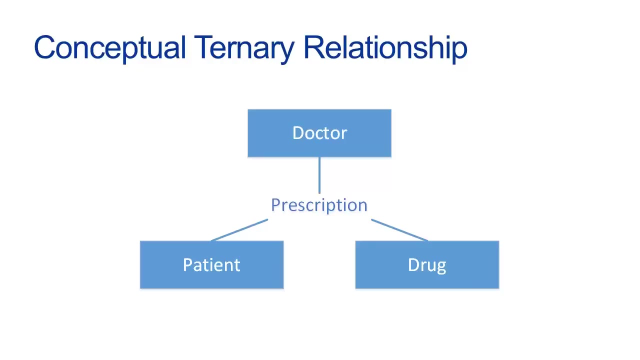 This is a binary relationship or a degree two relationship, and these types of relationships are the most common in entity relationship modeling. Here we see a conceptual ternary relationship. Recall that in a ternary relationship three different entities participate. In this case we have a doctor entity, a patient entity and a drug entity. 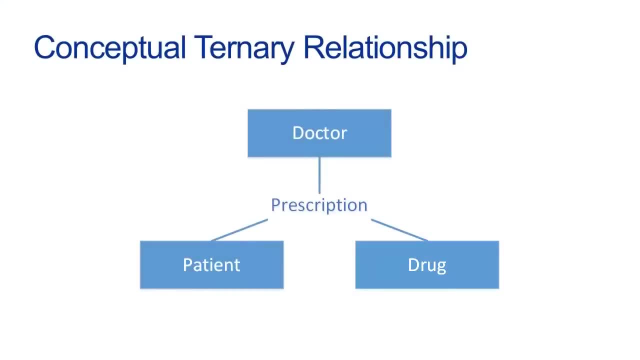 The intersection of these two entities is called a ternary relationship. These three entities, then, is a prescription, So a doctor writes a prescription which involves a patient and a specific drug. These three entities together, conceptually, are involved in a ternary relationship. 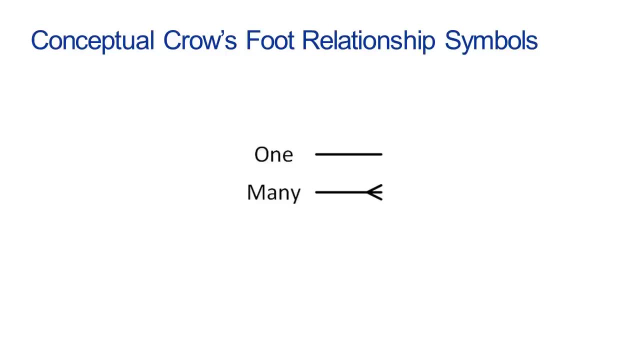 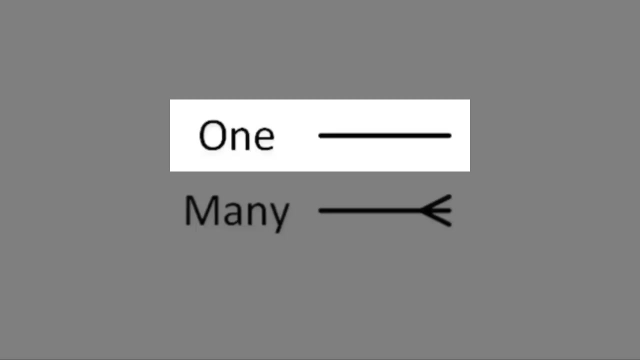 Next, let's expand the set of tools that we have available for describing the relationships between entities. We will begin by learning two simple symbols for describing conceptual relationships between entities. The first of these symbols is a simple line, and it is used to represent a conceptual one: relationship between entities. 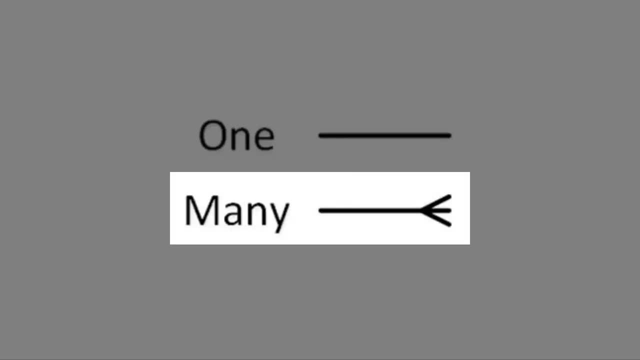 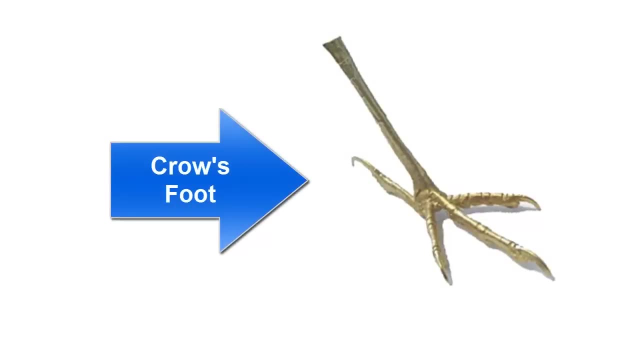 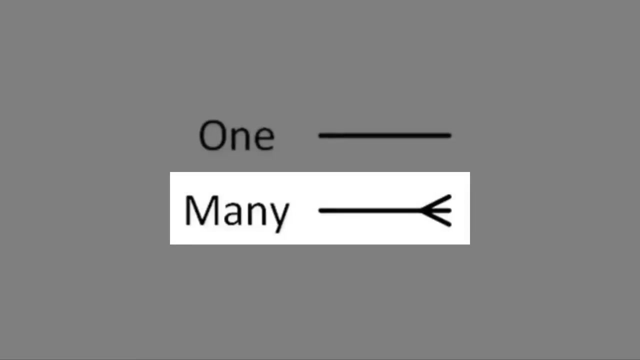 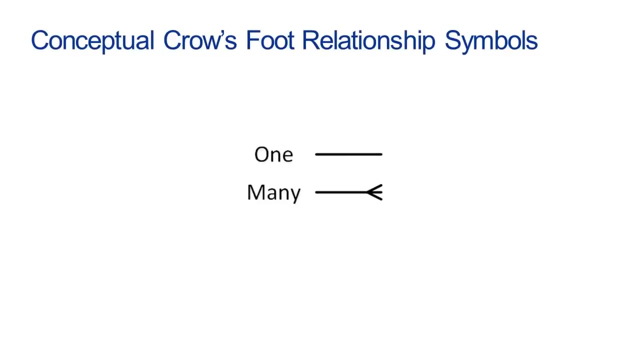 The second of these symbols is known as a crow's foot because it is supposed to look like the foot of a bird And we use this symbol to represent the conceptual notion of many. Let's see how these conceptual crow's foot relationship symbols might be implemented. 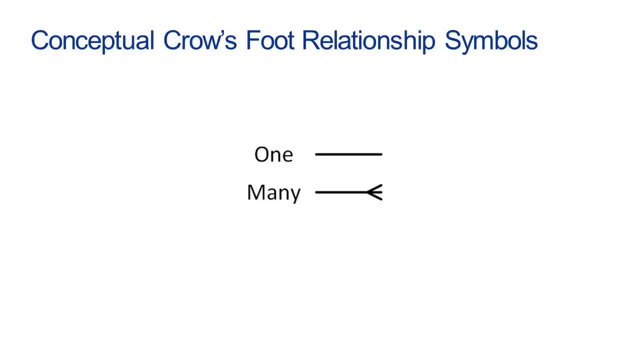 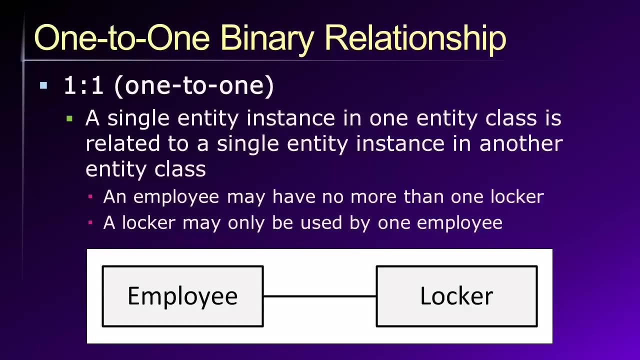 to describe relationships between entities with a little more detail. To begin, we can consider a conceptual one-to-one binary relationship. In a one-to-one relationship, an instance of one entity is related to one instance of another entity. Here we see an example of a one-to-one relationship between an employee entity and a locker entity. 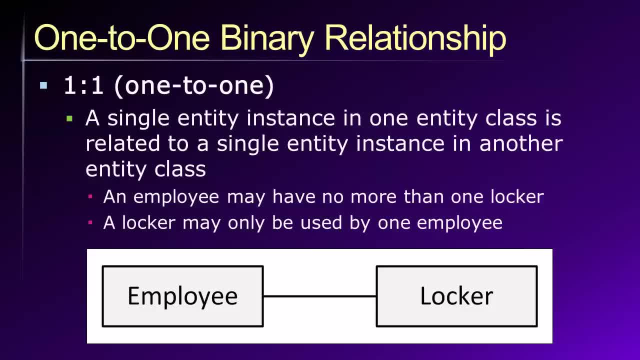 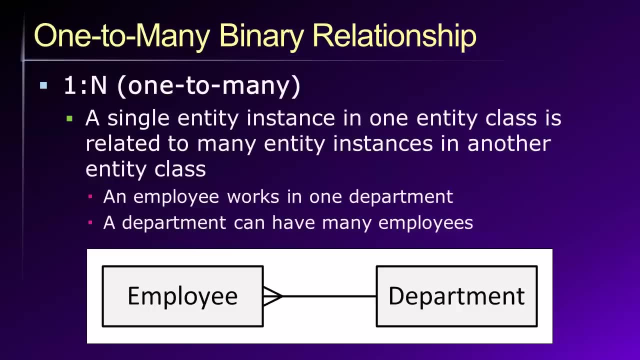 So we might imagine that an employee is assigned to exactly one locker and a locker can be assigned to just one employee. This is a one-to-one relationship. Next, we can consider a one-to-many relationship. I should note that one-to-many relationships are by far the most common types of binary relationships. 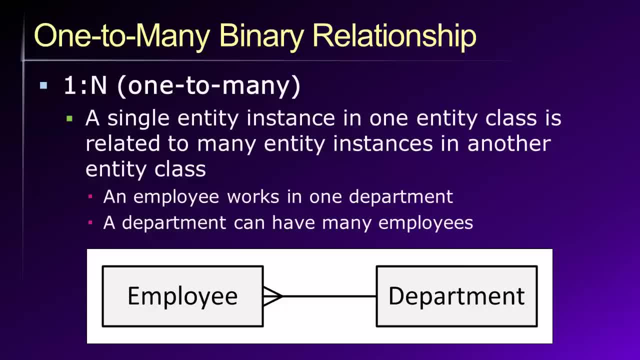 I should note that one-to-many relationships are by far the most common types of binary relationships. I should note that one-to-many relationships are by far the most common types of binary relationships. In a one-to-many relationship, a single instance of one entity is conceptually related to many instances of another entity. 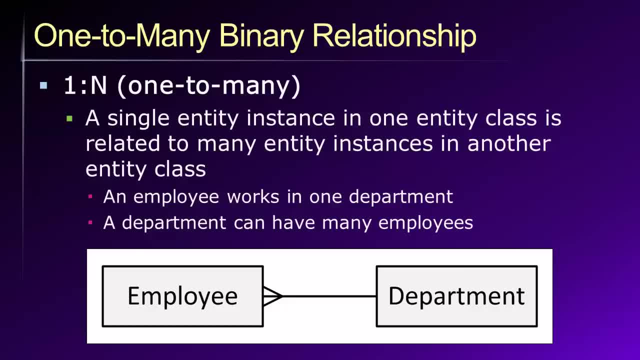 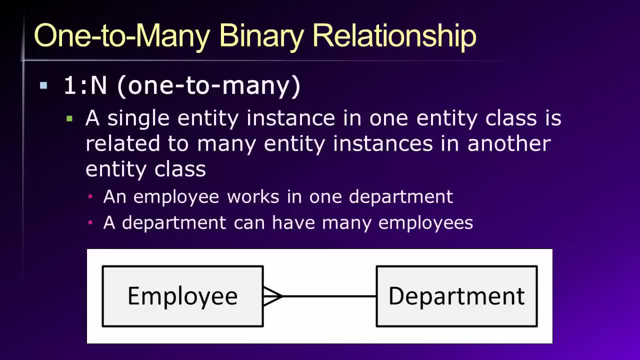 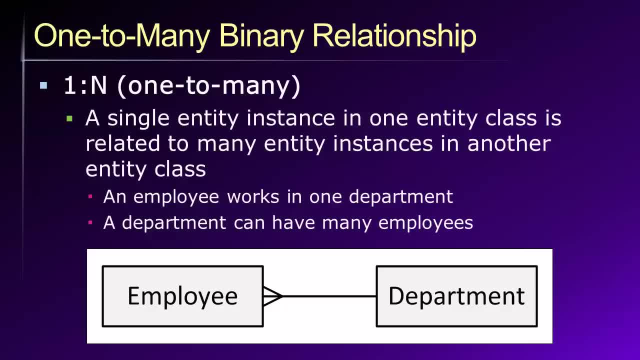 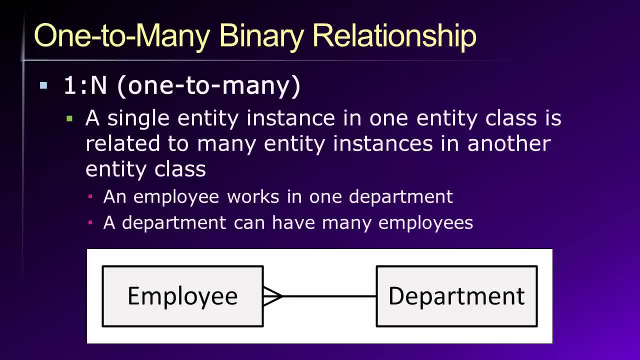 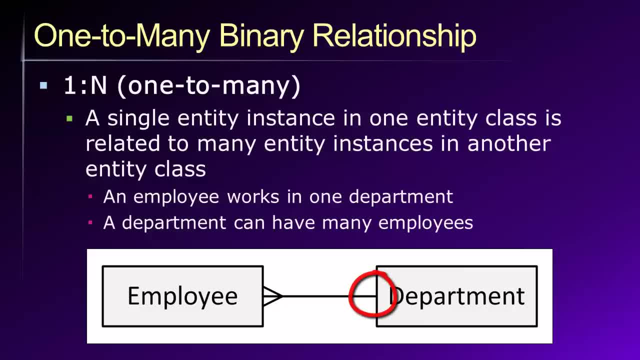 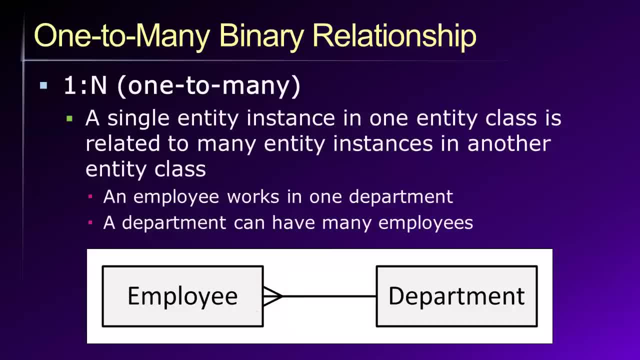 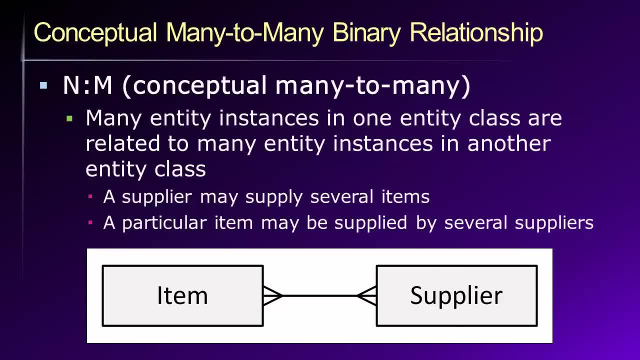 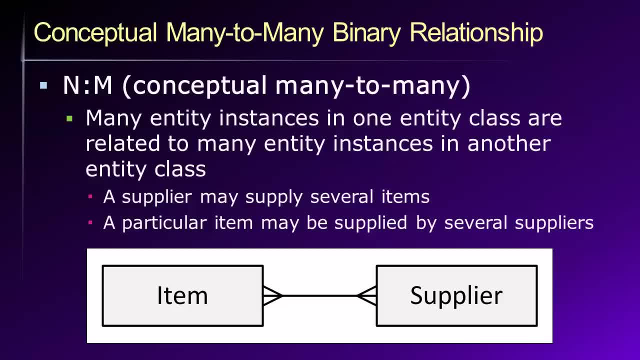 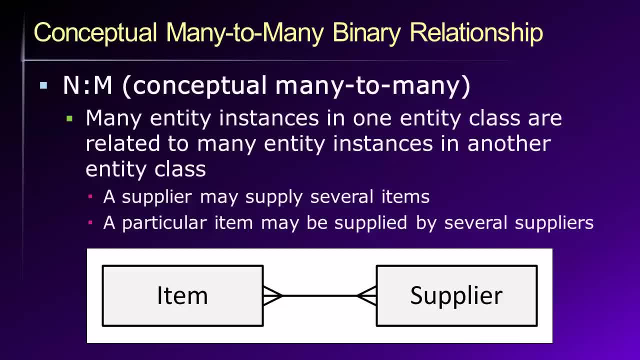 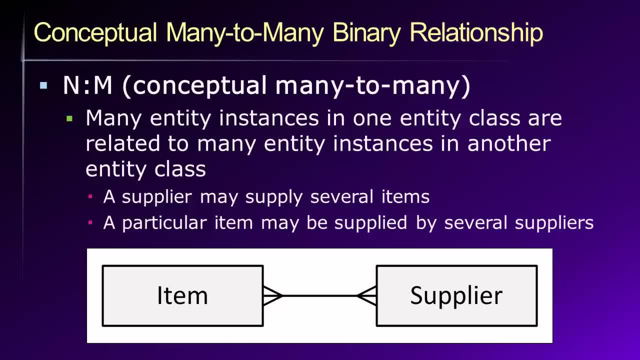 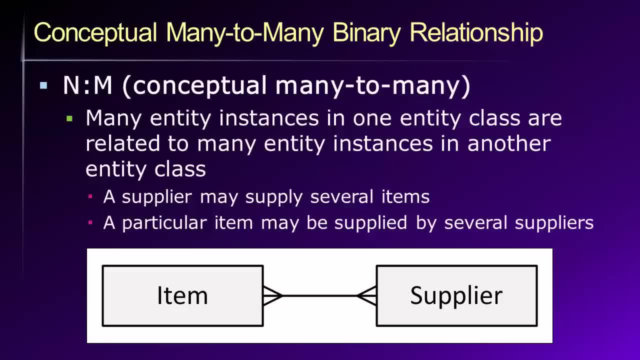 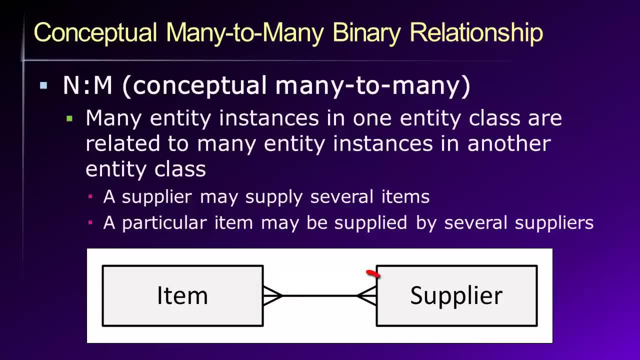 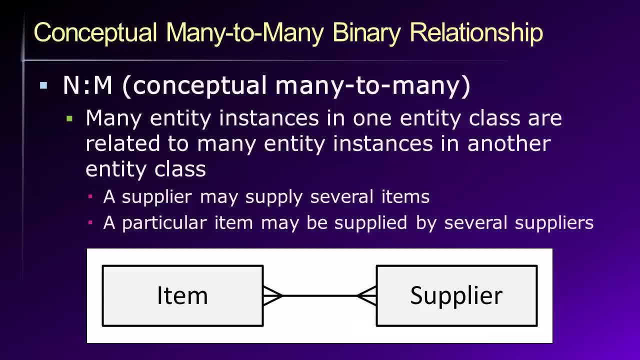 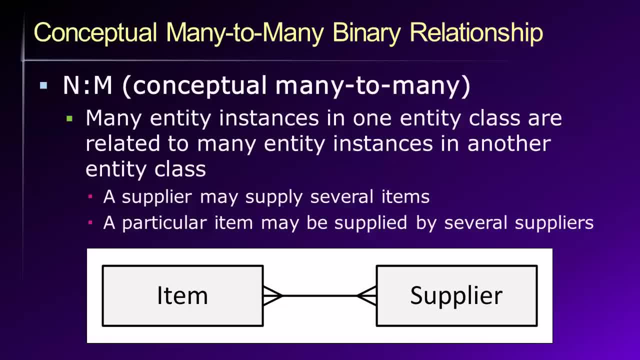 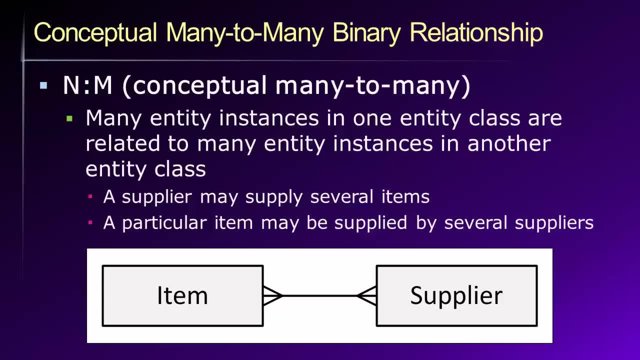 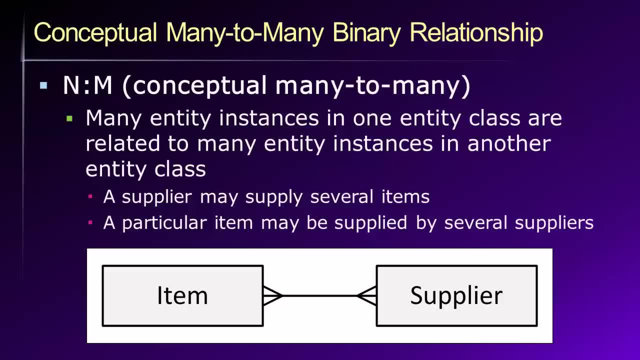 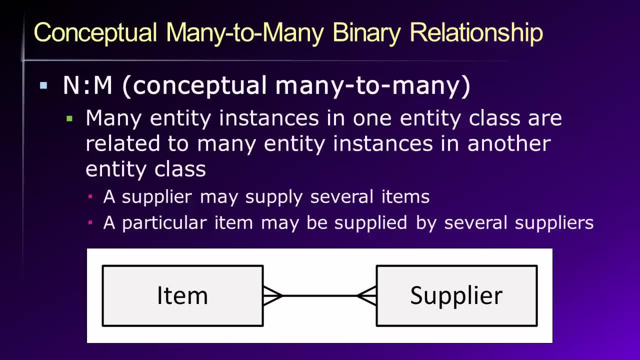 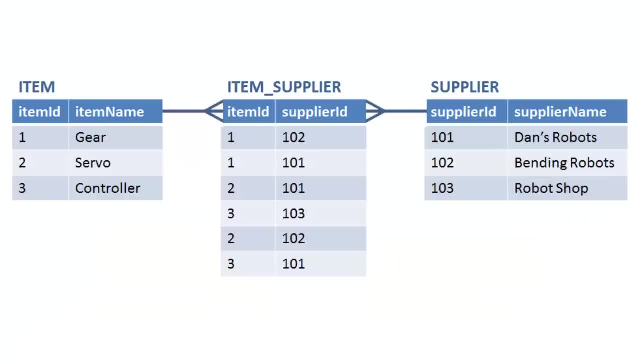 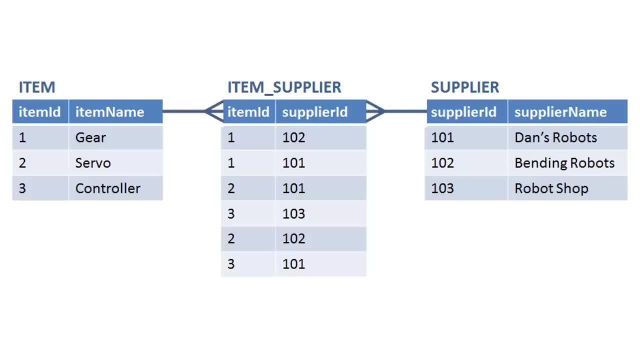 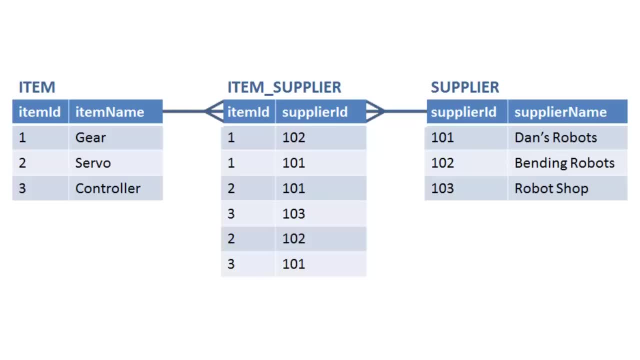 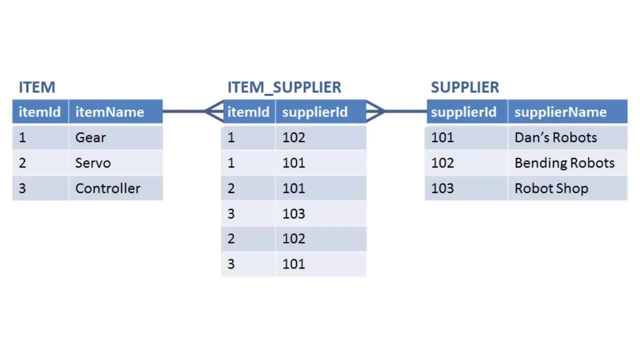 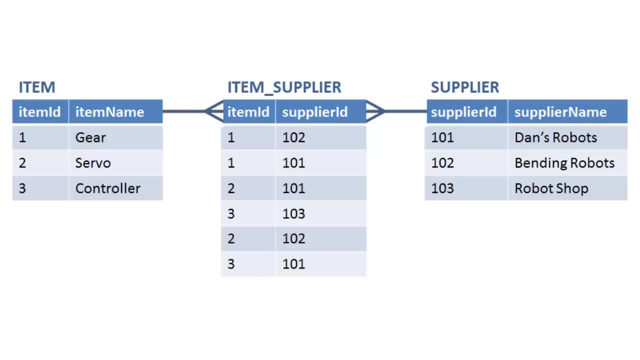 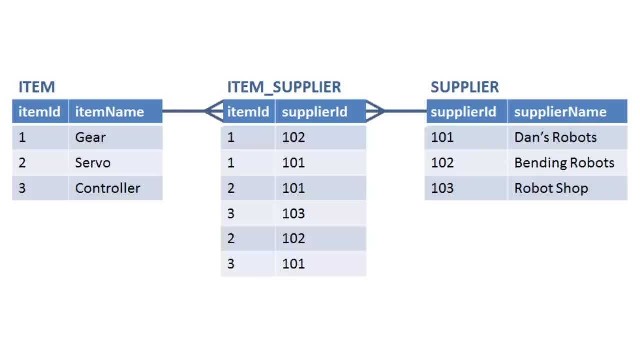 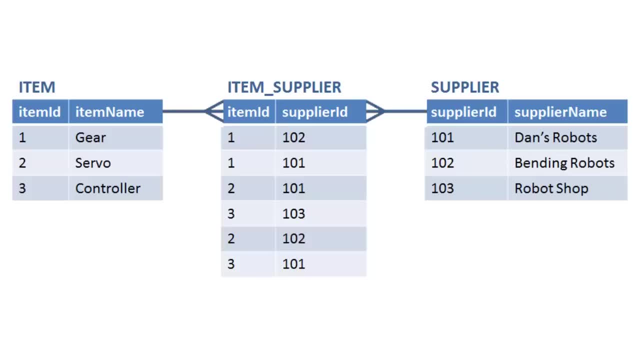 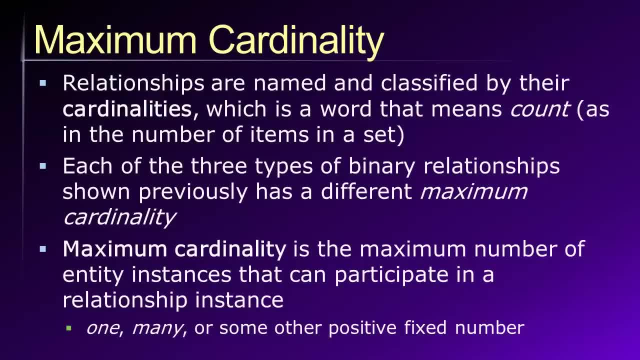 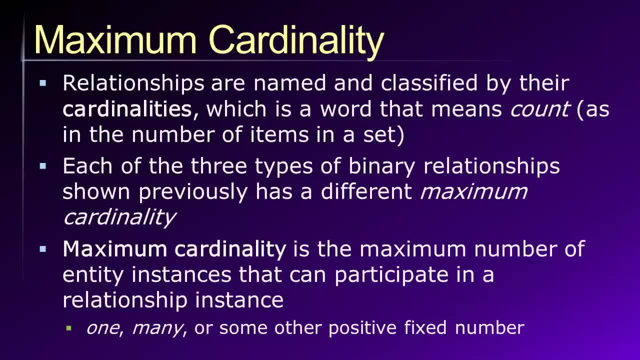 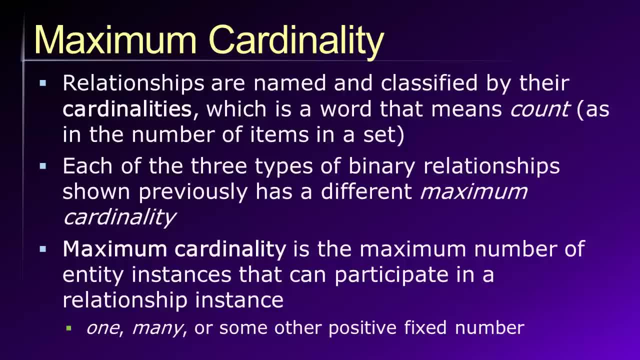 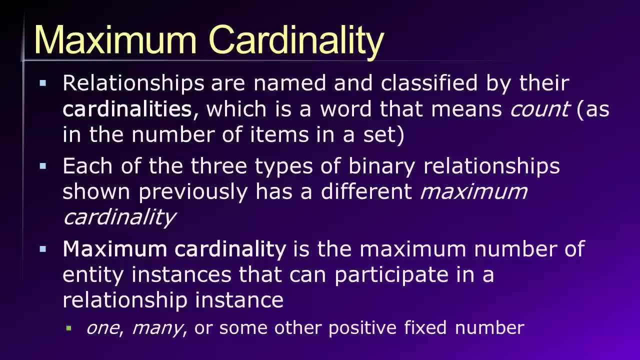 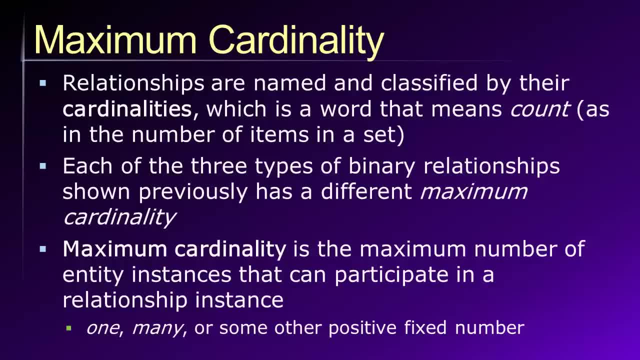 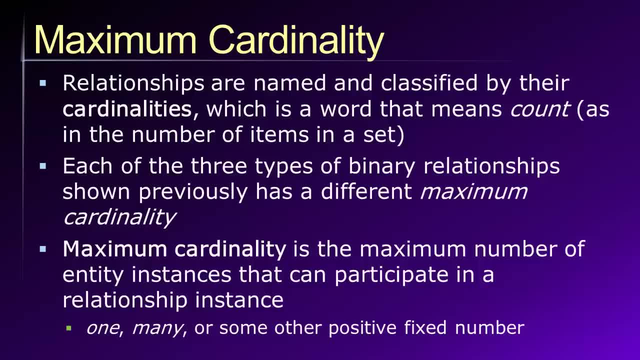 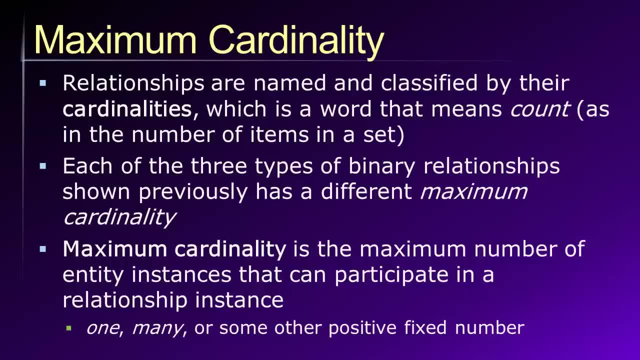 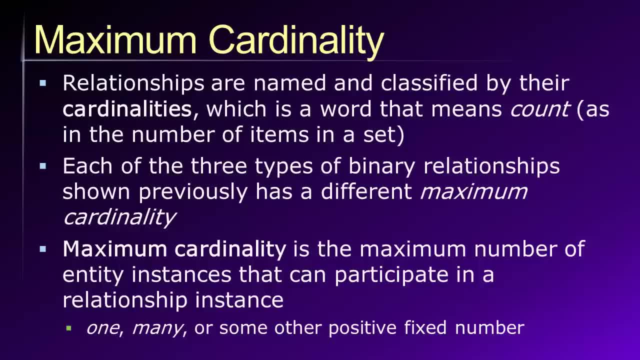 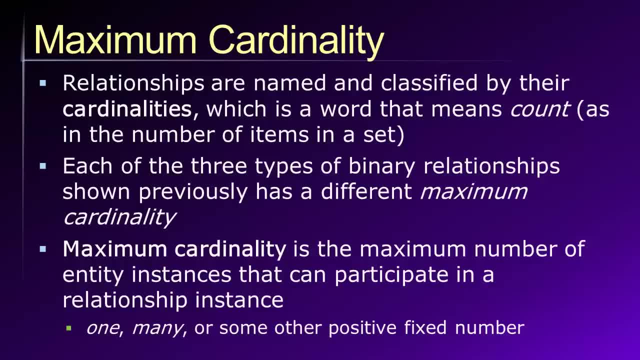 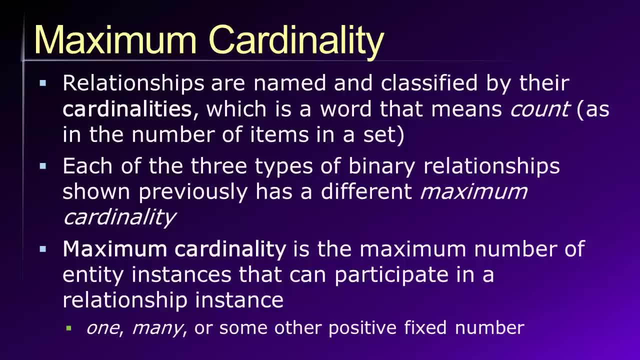 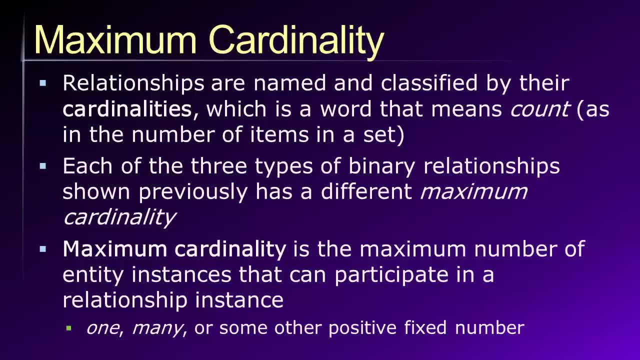 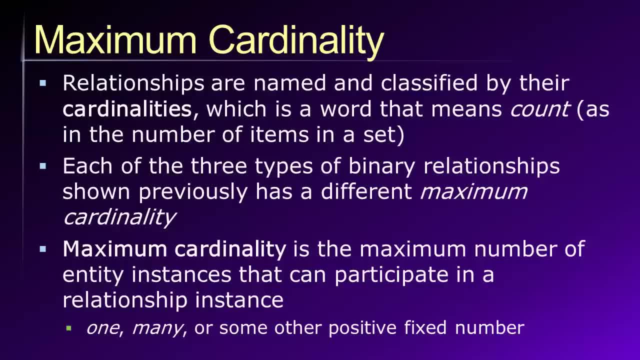 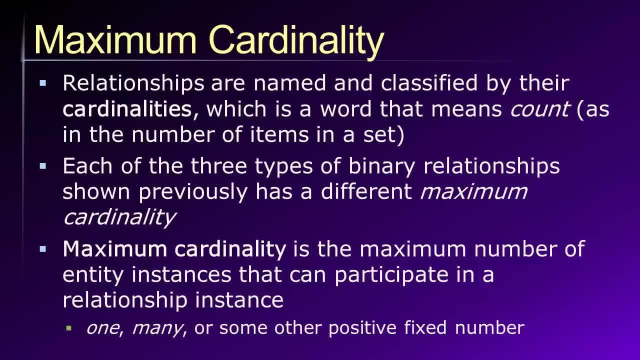 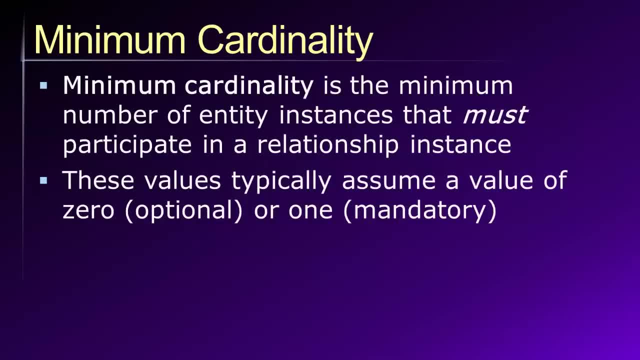 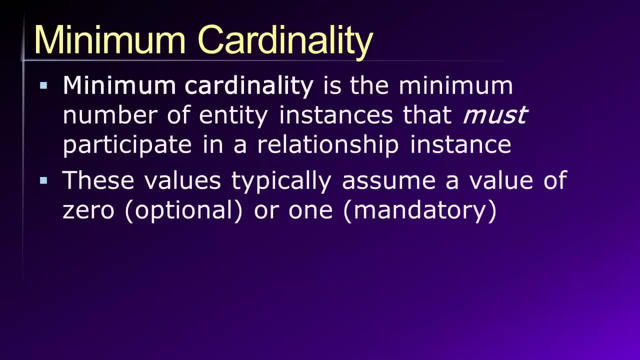 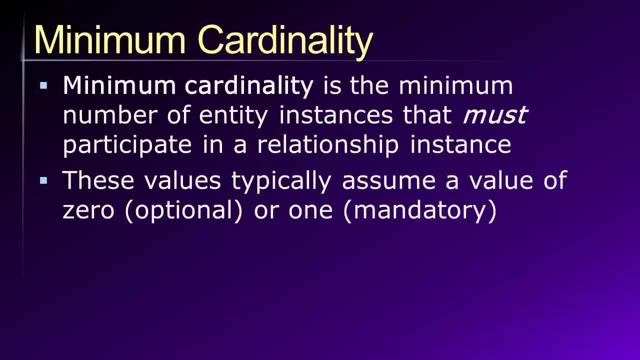 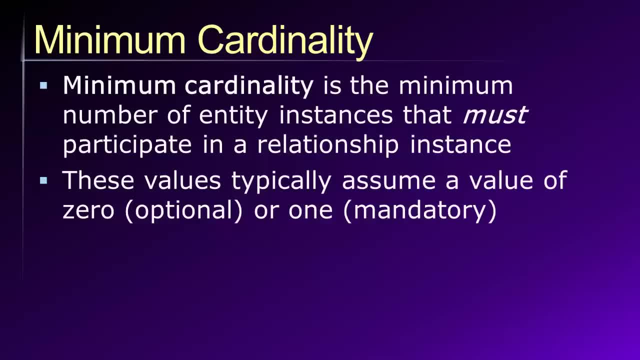 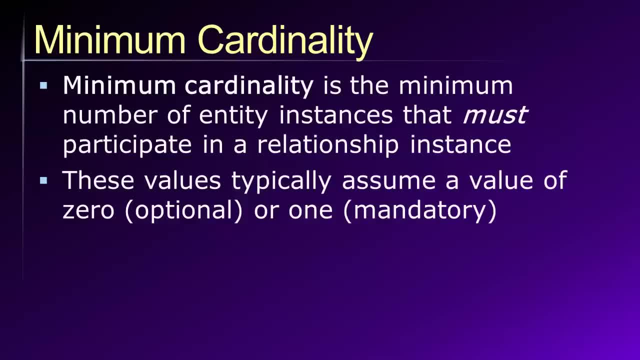 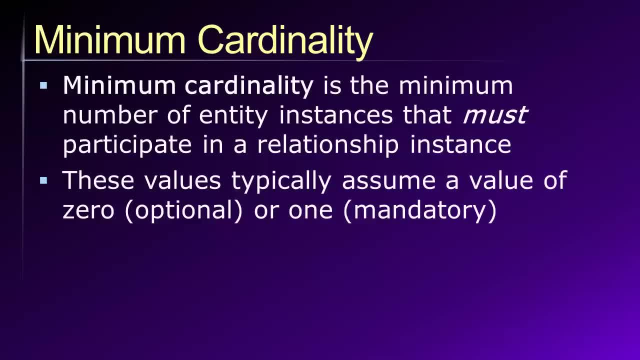 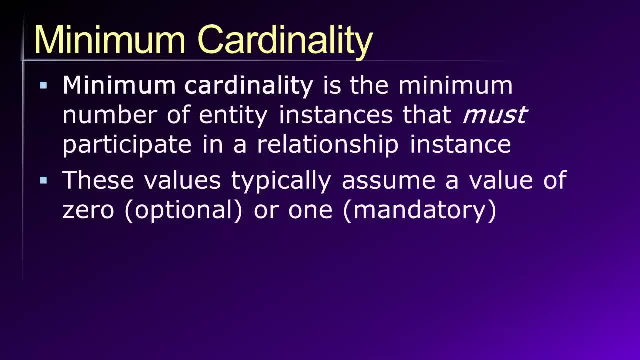 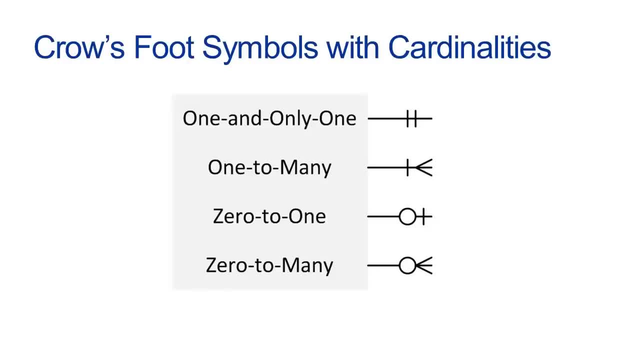 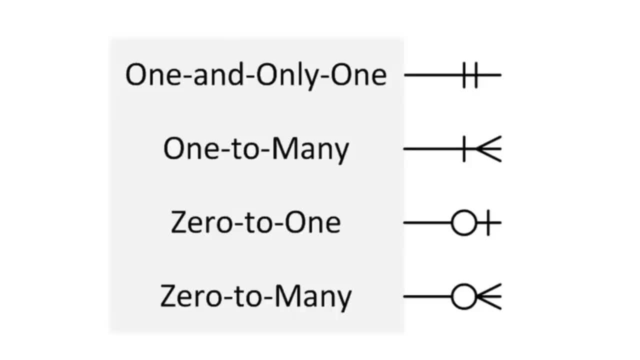 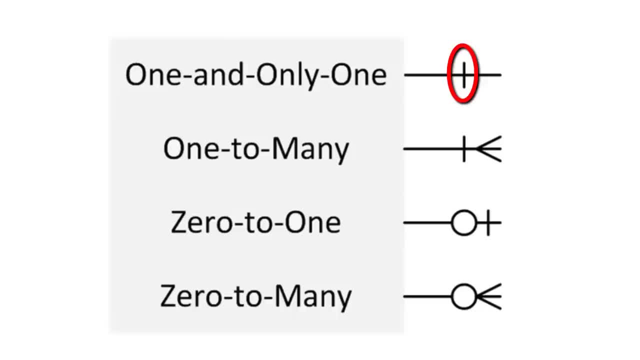 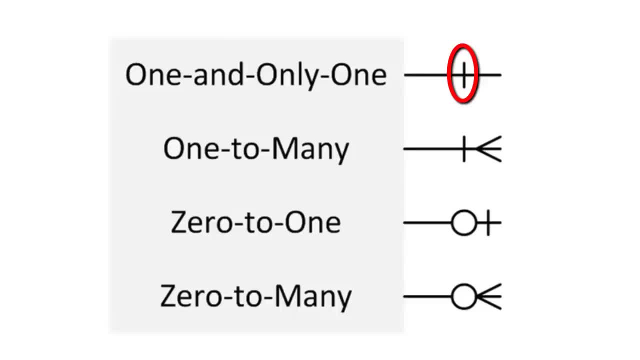 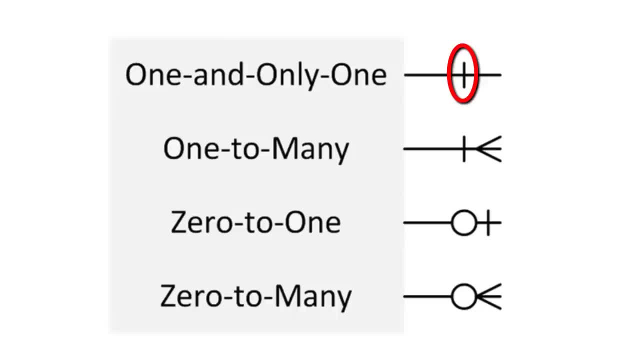 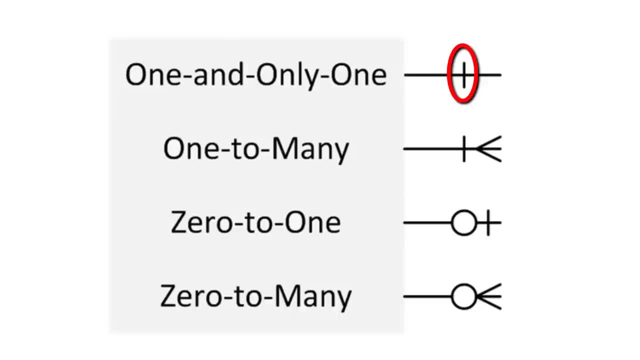 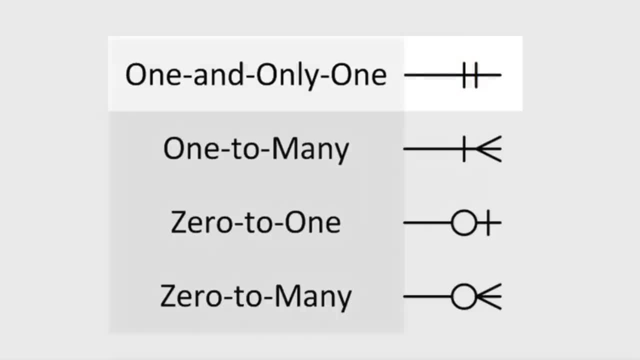 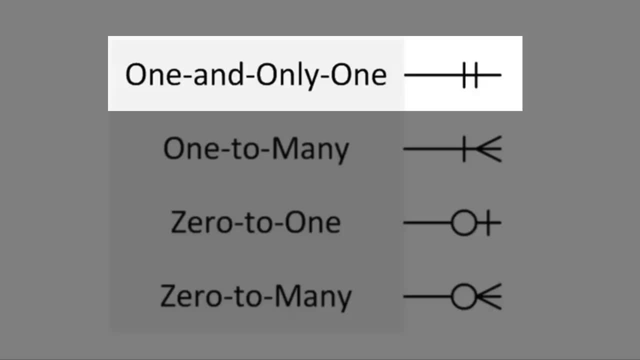 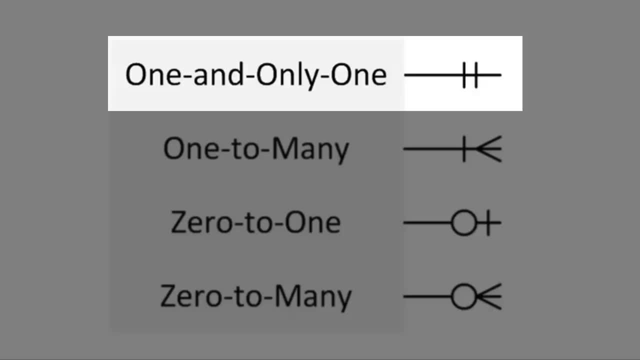 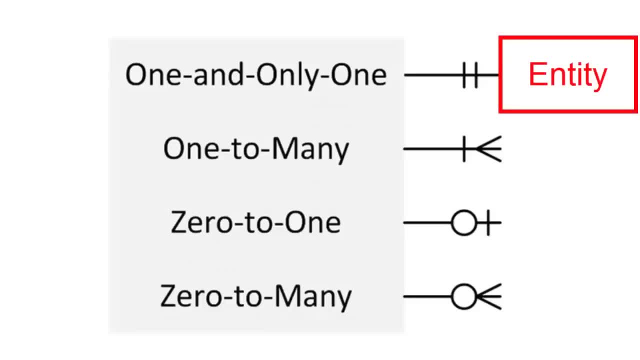 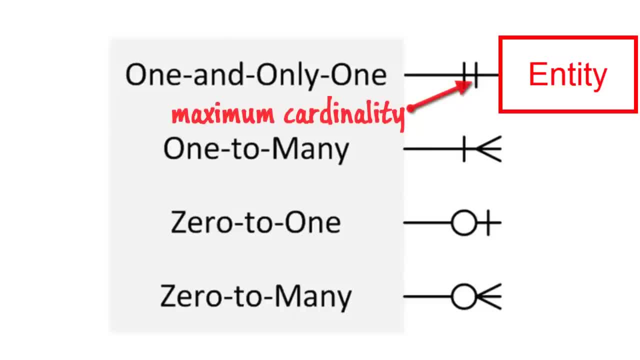 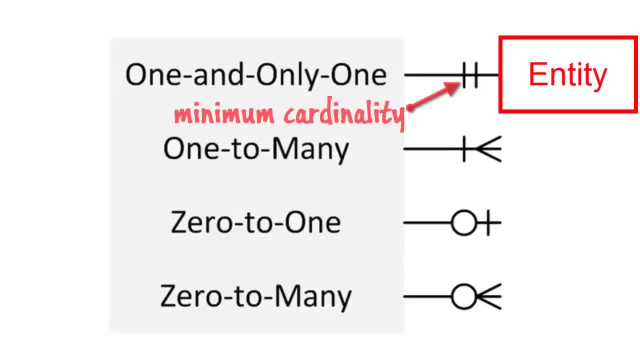 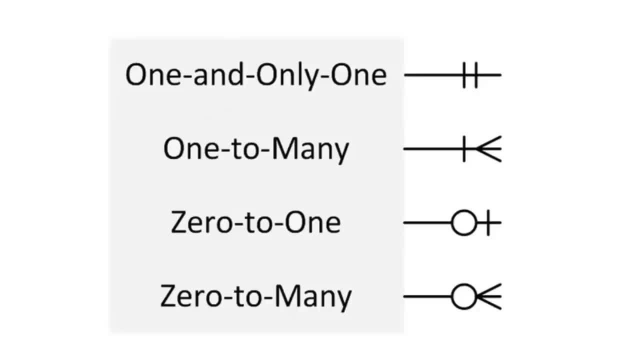 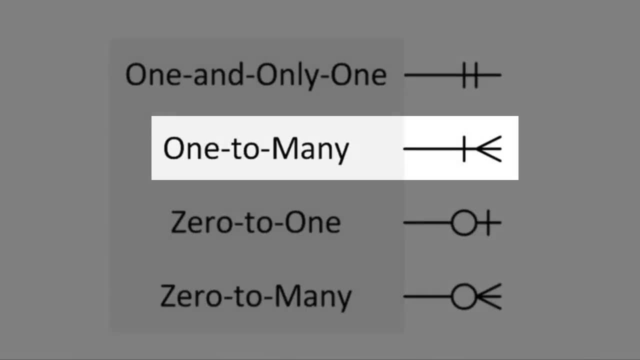 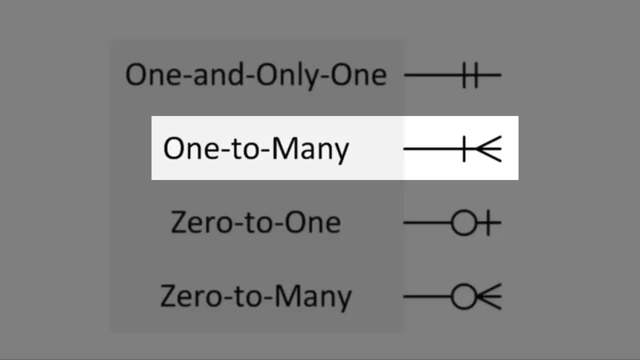 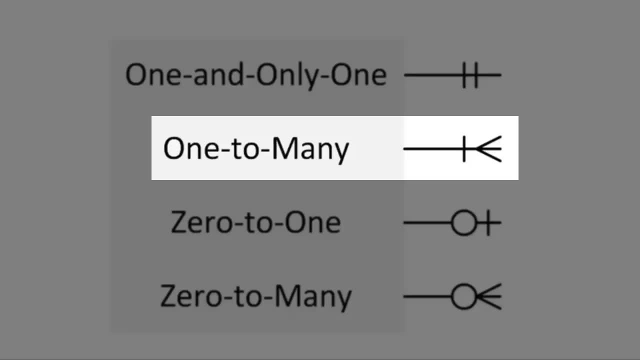 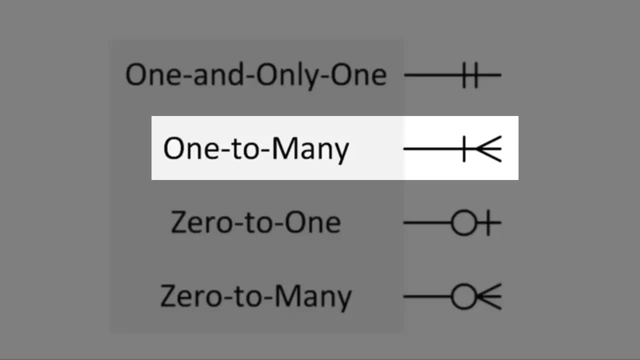 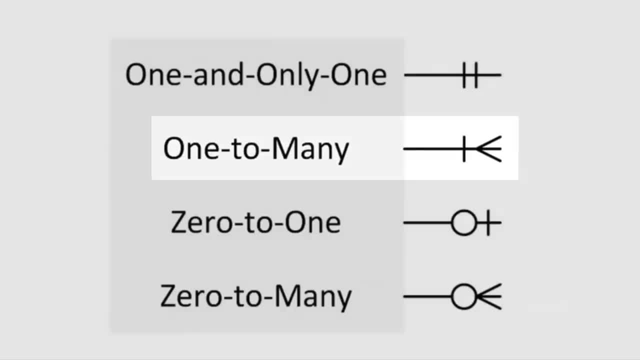 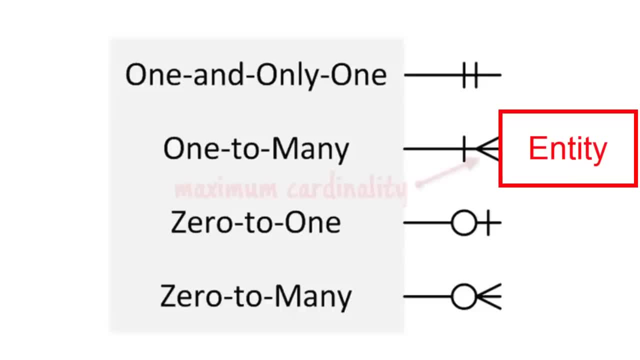 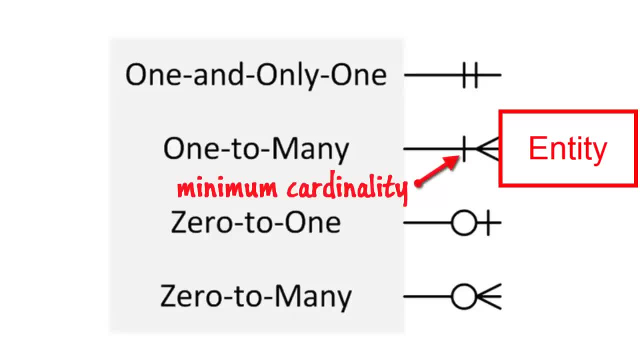 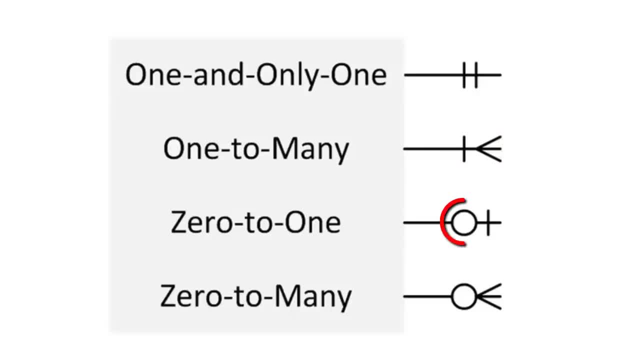 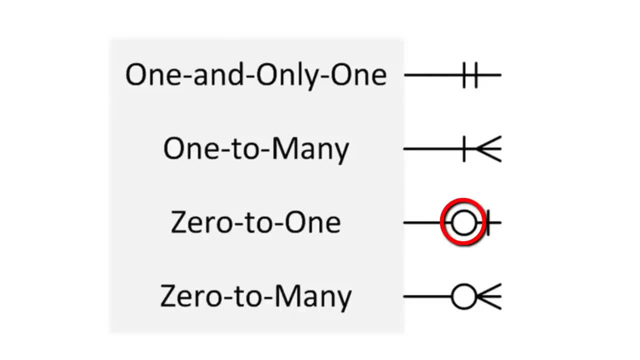 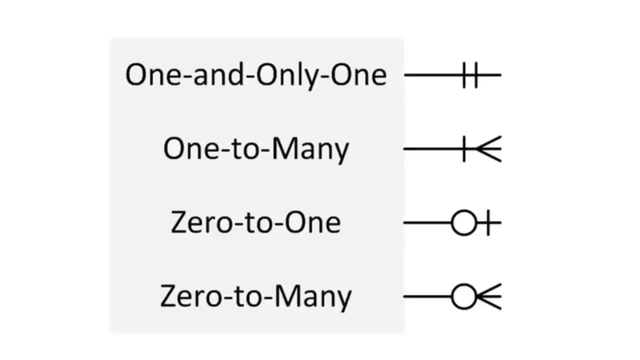 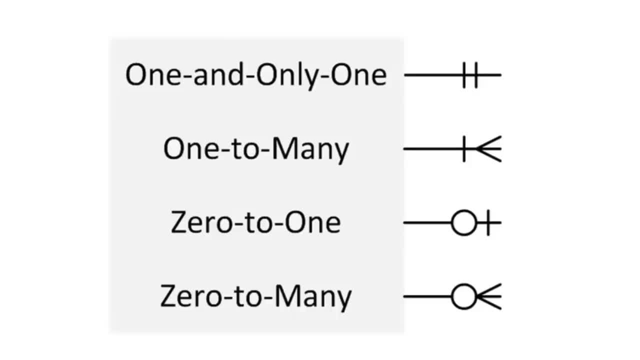 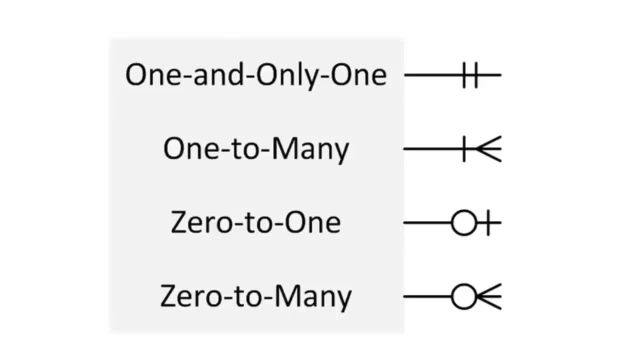 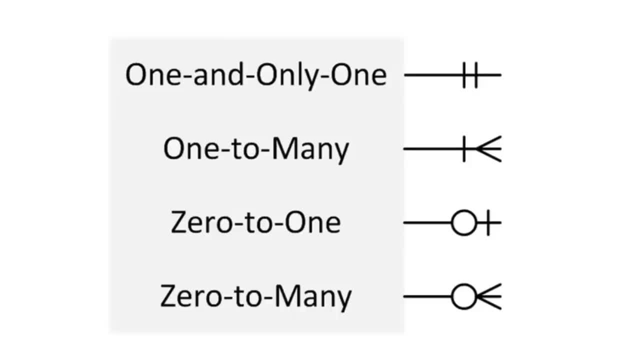 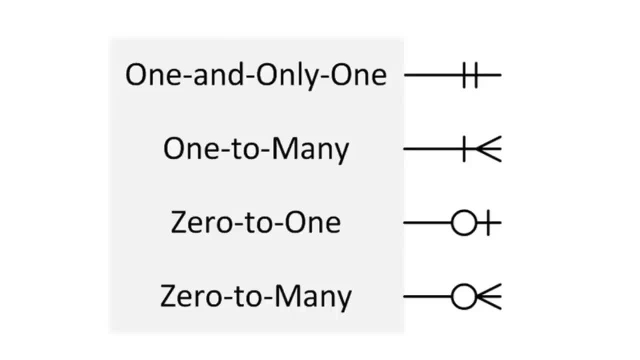 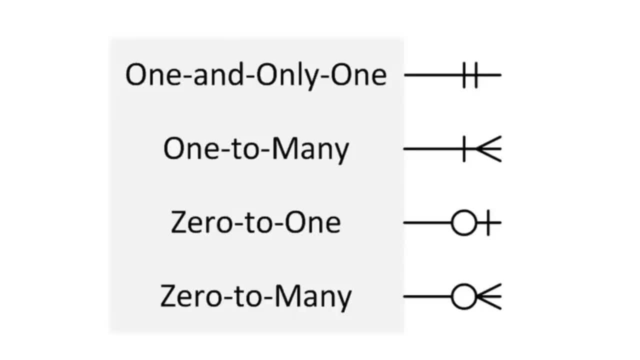 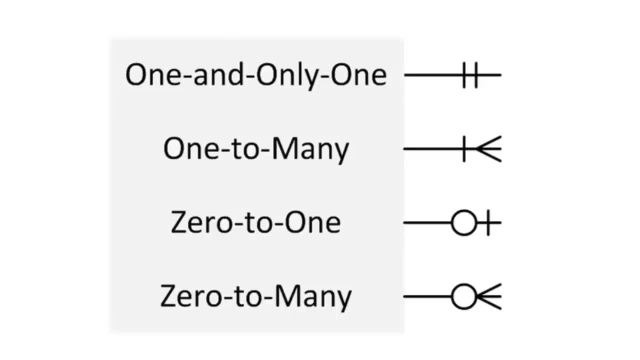 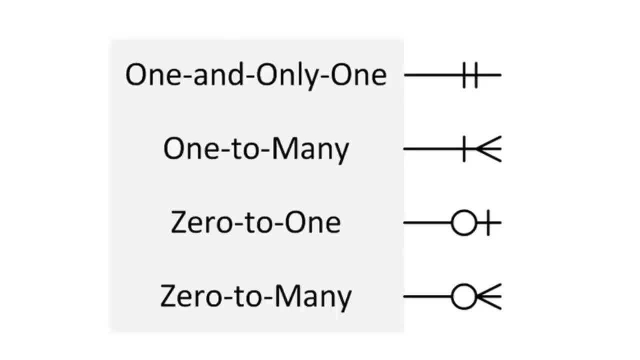 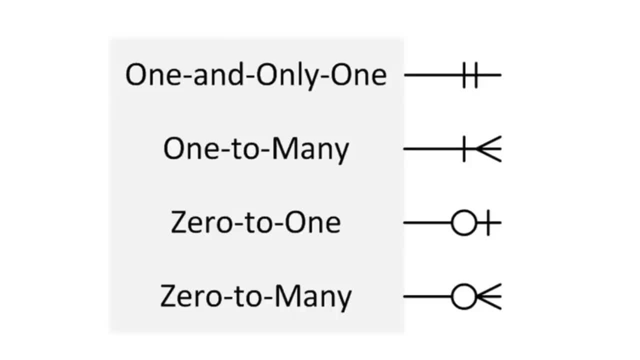 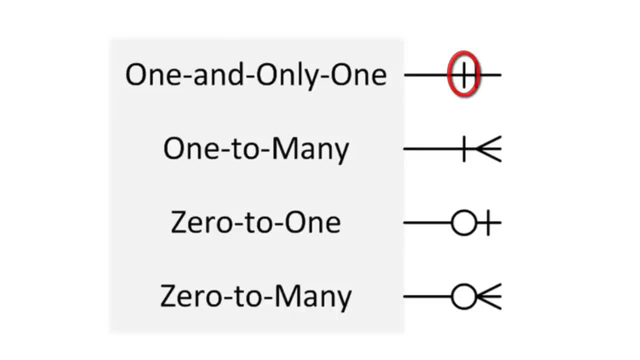 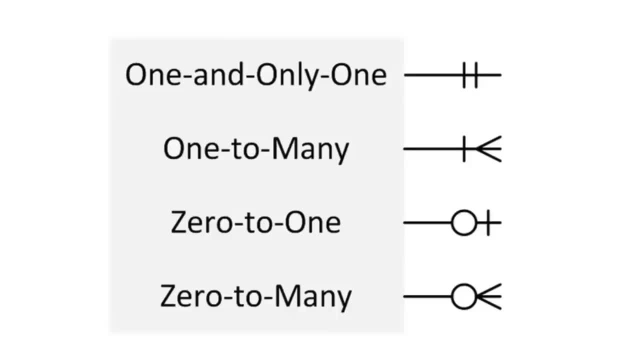 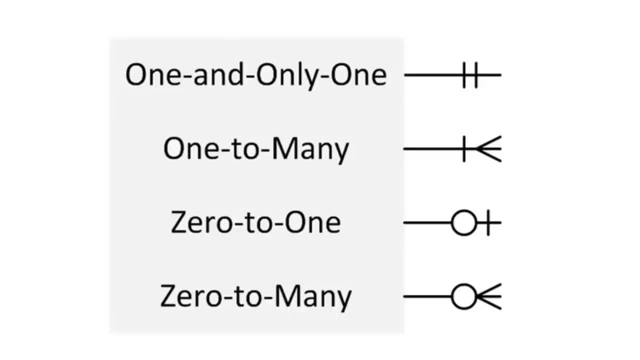 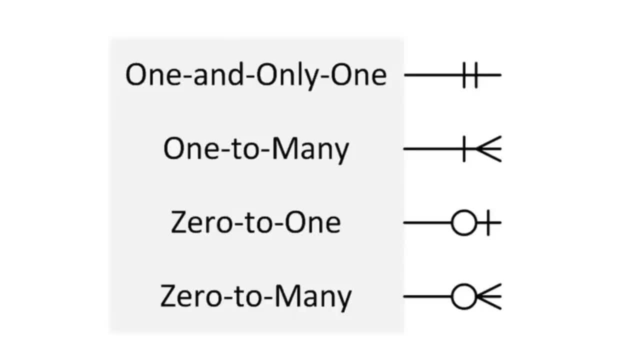 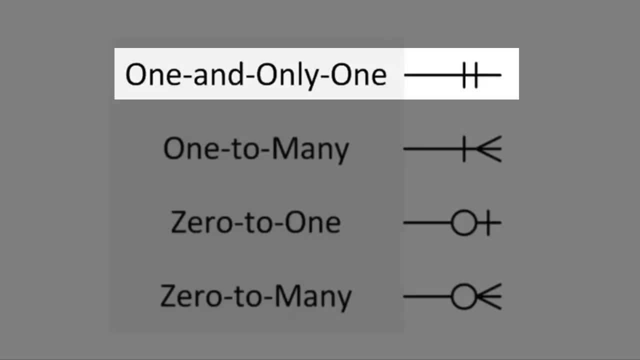 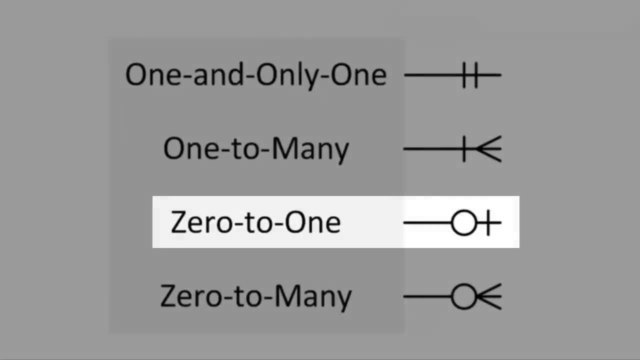 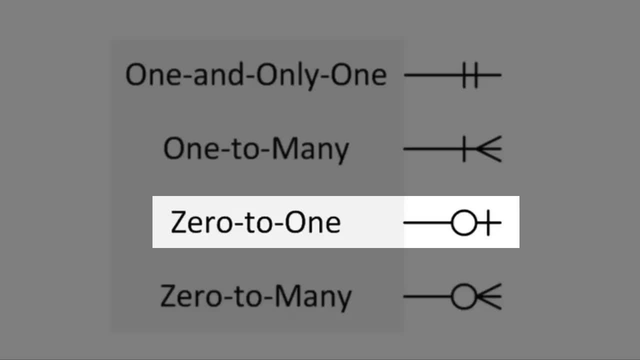 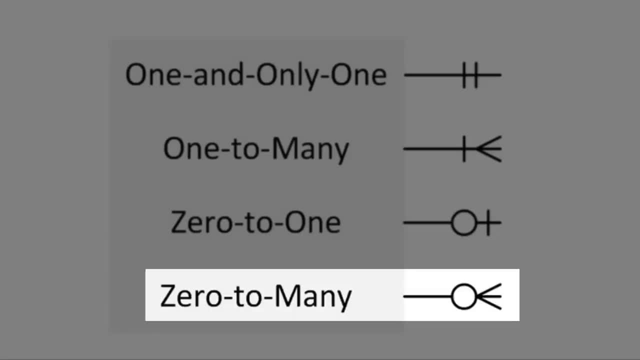 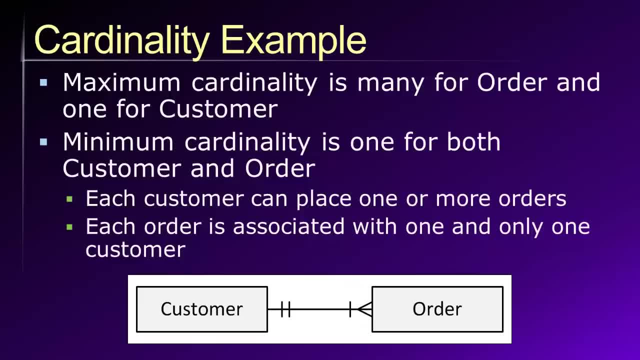 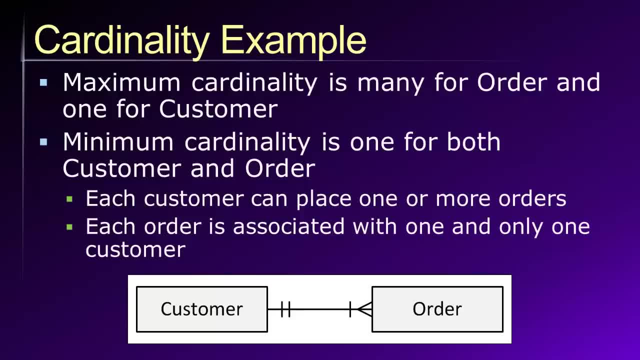 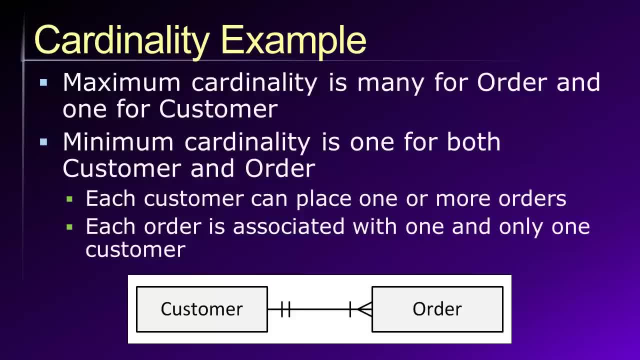 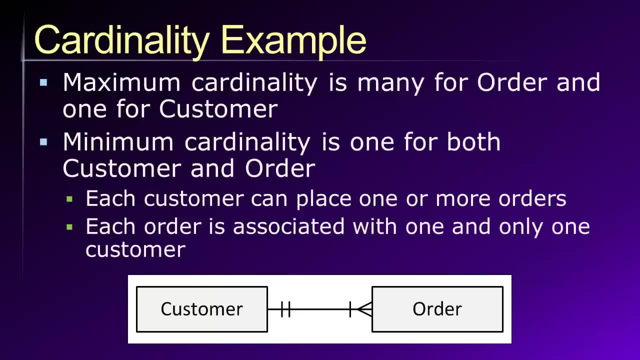 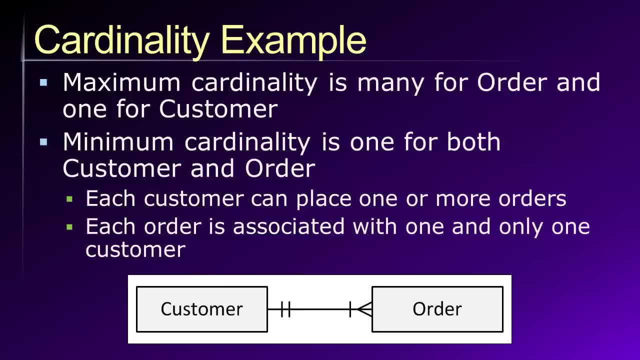 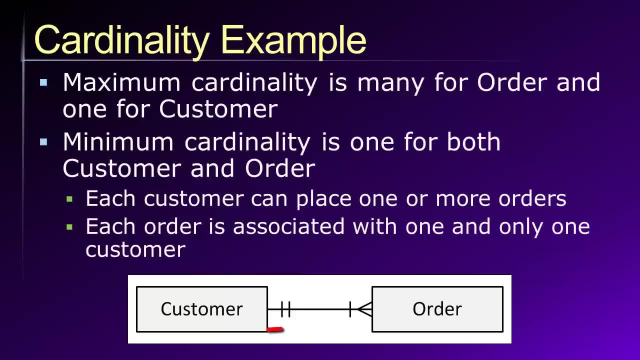 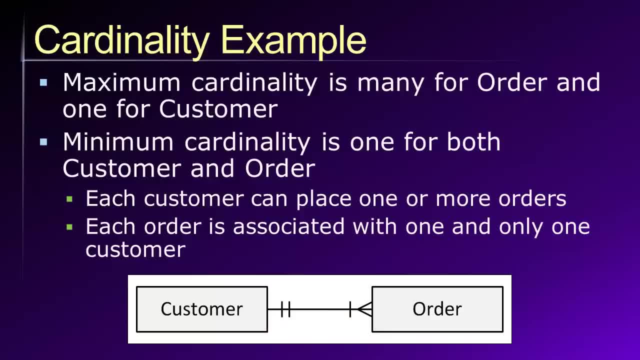 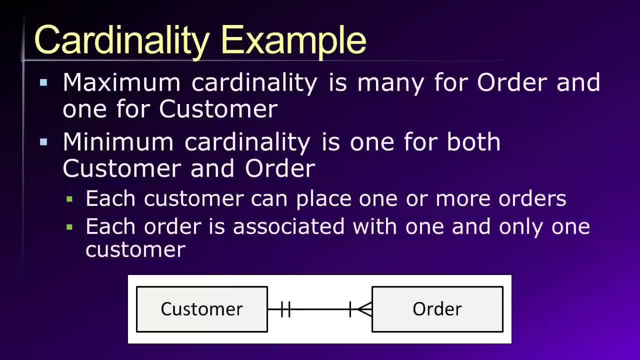 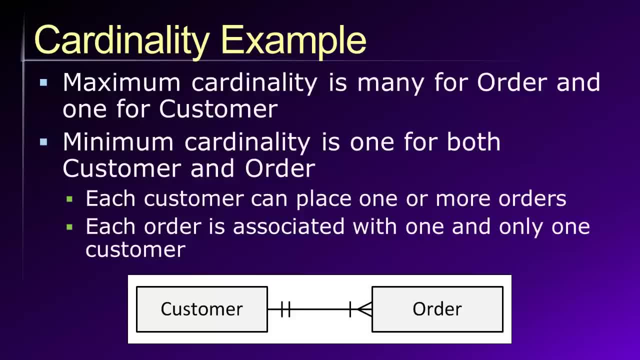 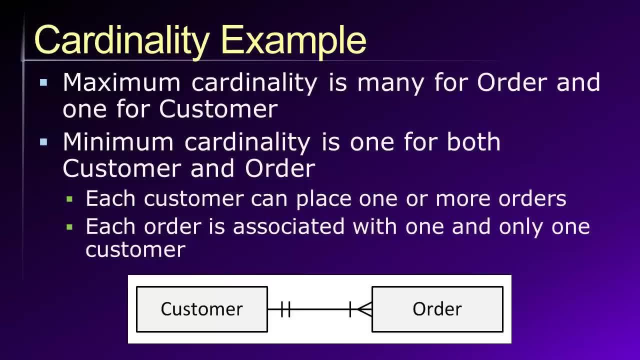 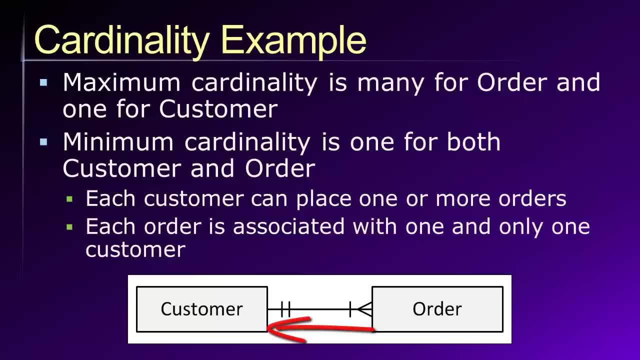 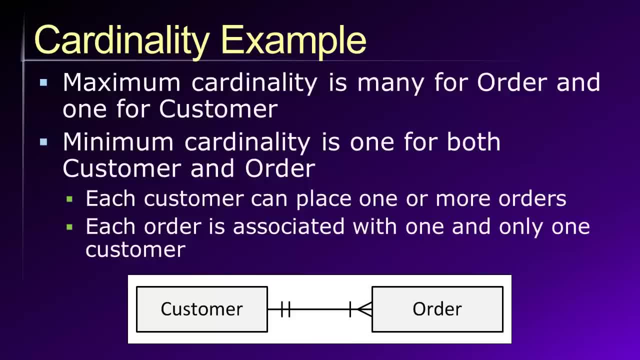 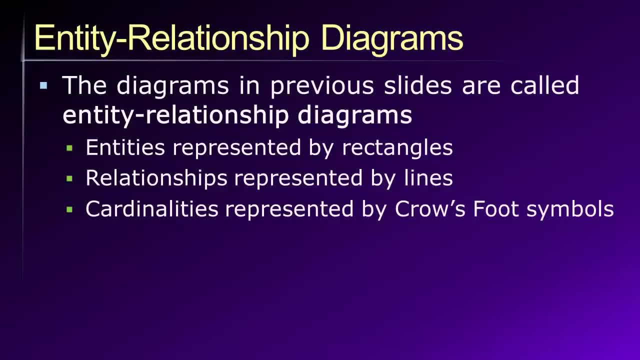 that we have been seeing on the previous slides are what are known as entity relationship diagrams. They are graphical ways of describing relationships among the various entities that will eventually become a part of the database. In these entity relationship diagrams, our entities, or our tables, if you will. 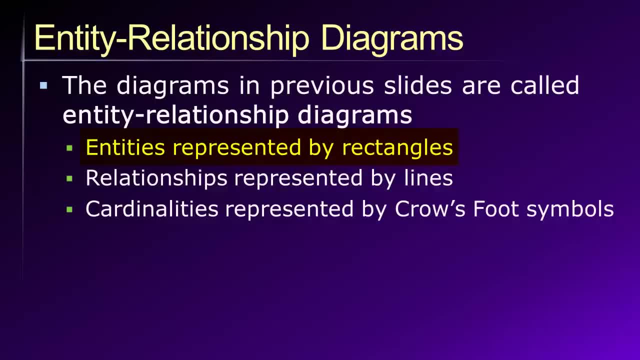 are represented by rectangles. Inside of those rectangles you will see the names of the entities and potentially, the attributes that together define the entity. Entity relationship diagrams also depict relationships And these are shown by using lines that interconnect. These are entities And, as we saw on the previous slide, 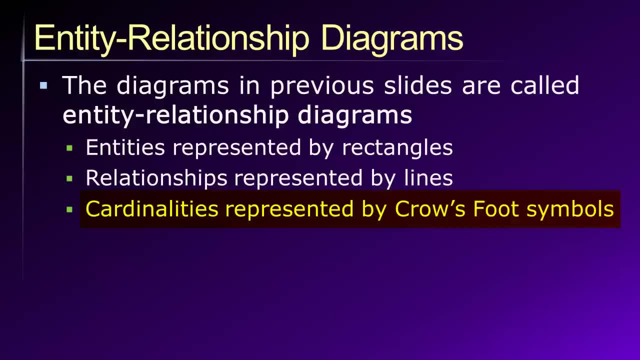 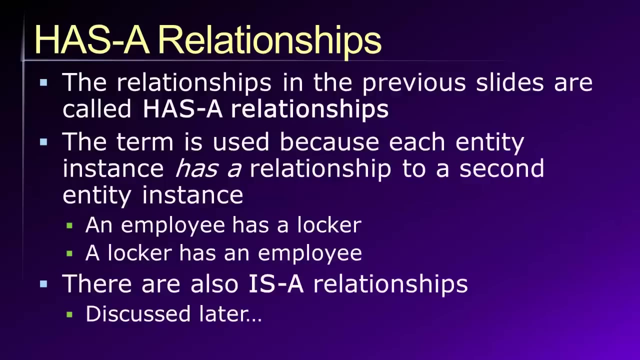 the specific nature of those relationships is depicted using our cardinality symbols. Specifically, we use crow's foot symbols in order to provide specific details about the nature of the relationship between two entities. All of the examples that I've shown you today and all of the examples that we've seen today, 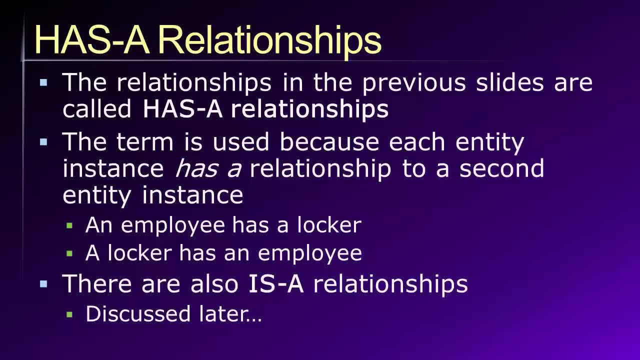 can be thought of as what we would call has-a relationships, And this term is used because an entity has a relationship with some other entity. For example, an employee has a locker, A department has an employee. There are other types of relationships between entities. 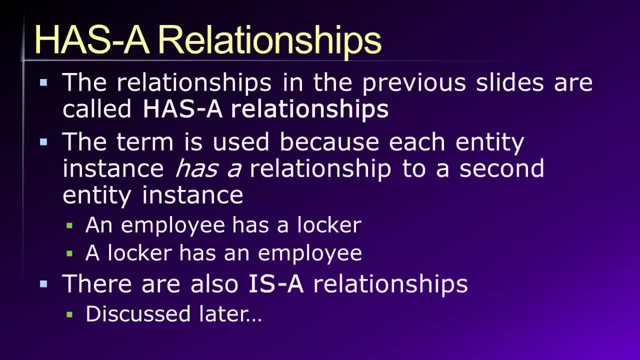 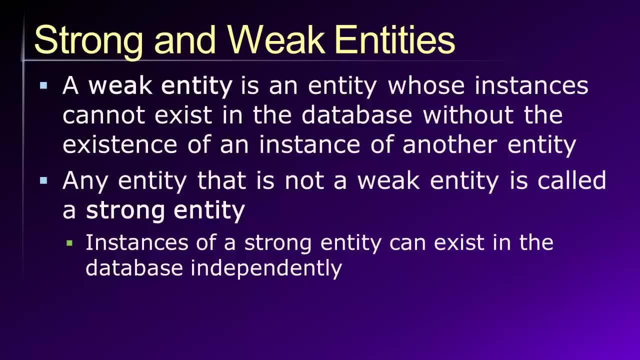 which are called is-a relationships, And we will discuss these a little later. First, however, let's talk about strong and weak entities. To begin, a weak entity is an entity whose instances cannot exist in the database unless they are related to an instance. 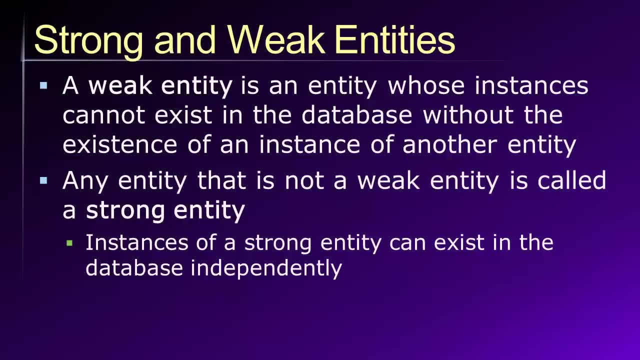 in another entity. By contrast, a strong entity is an entity whose instances can exist independently. They do not rely on the existence of instances of any other entity in order to be able to exist. They can be added to the database independently. Consider, for example, the relationship: 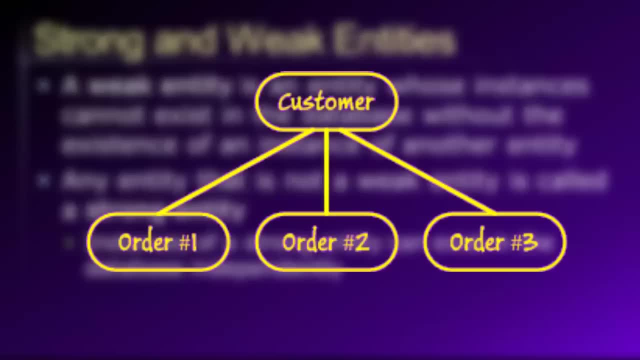 between two entities: A customer entity and an order entity. New customers can be added to the database without any additional information being required to exist in any other entities. However, we cannot add an order to the database unless that order is associated with an existing customer. 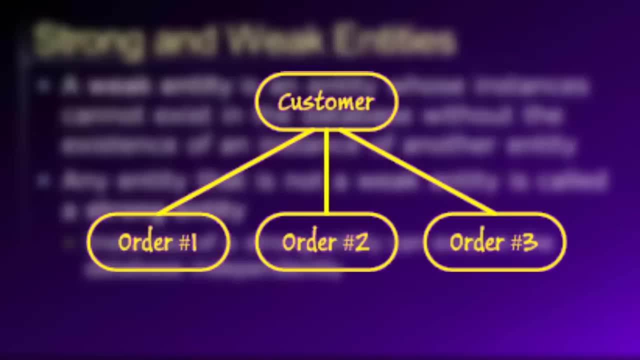 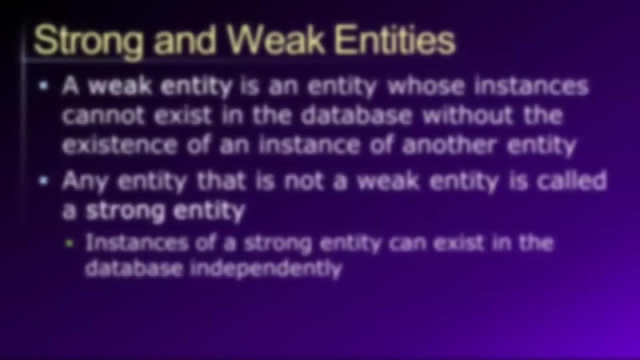 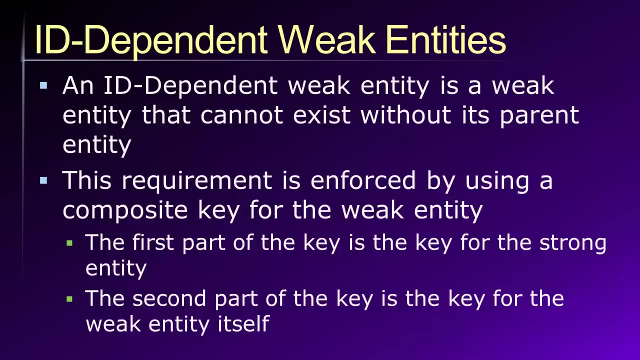 In this case. in this example, a customer would be a strong entity, whereas an order would be a weak entity. Beyond the distinction between strong and weak entities, we also need to note that there are two different types of weak entities. These are ID-dependent weak entities. 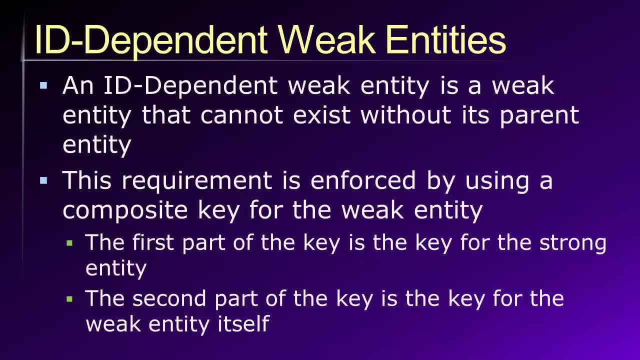 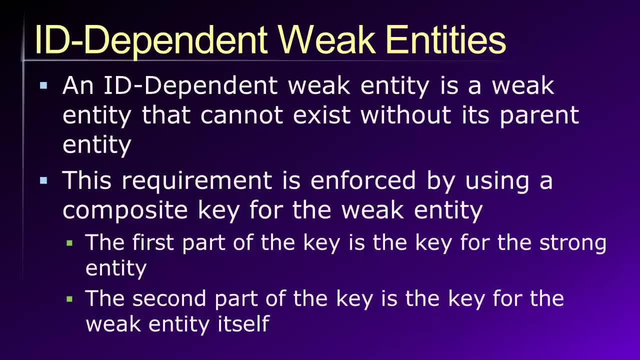 Another way of saying that is, the ID dependent weak entity will have as part of its primary key the primary key of its parent entity. In this way, the database will enforce the constraint that instances of the ID dependent weak entity cannot exist without being associated. 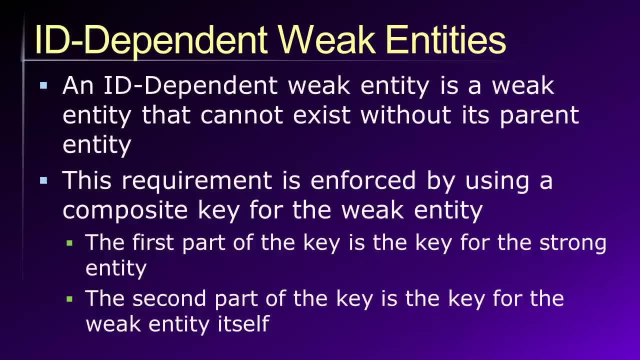 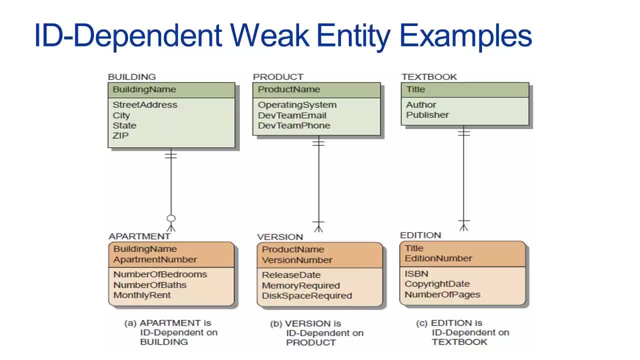 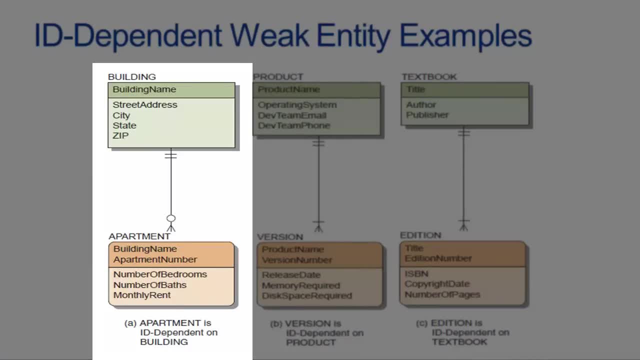 with an instance of its parent entity. Here we see some examples Of these ID dependent weak entity relationships. In the first case, we may have a parent entity which we will call building and a child entity which we will call apartment. 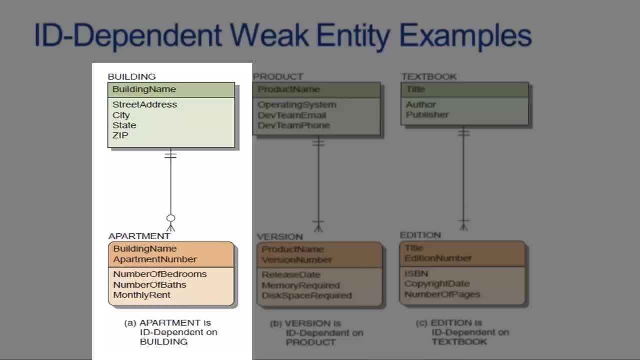 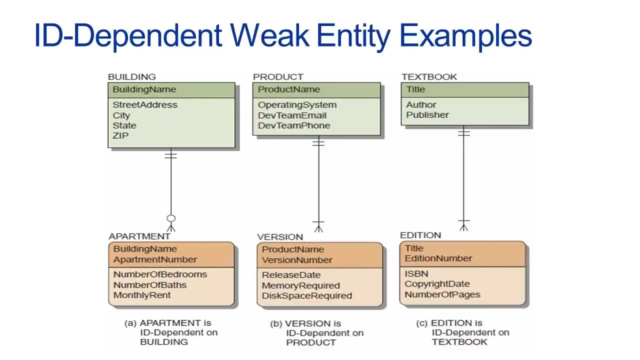 In this model, an apartment cannot exist without belonging to a building, And this constraint is enforced by making the building name a component of the primary key for ID Apartment. If the relationship between a strong entity and a weak entity is ID dependent, then we call that relationship. 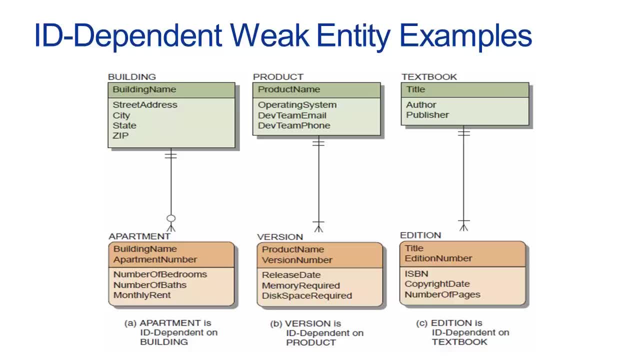 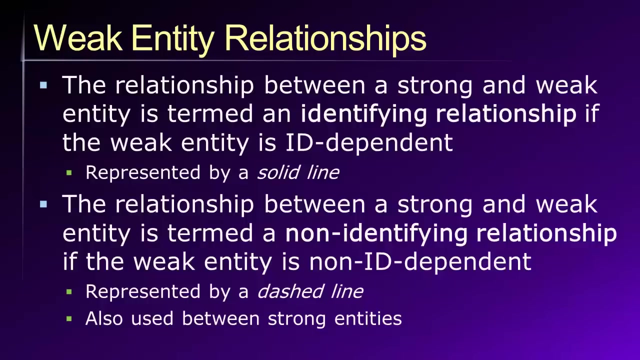 an identifying relationship And this can be seen graphically in entity relationship models by the use of a solid relationship line connecting the strong entity to the weak entity. So just to reiterate, ID dependent weak entity relationships are known as identifying relationships. These are represented using a solid line. 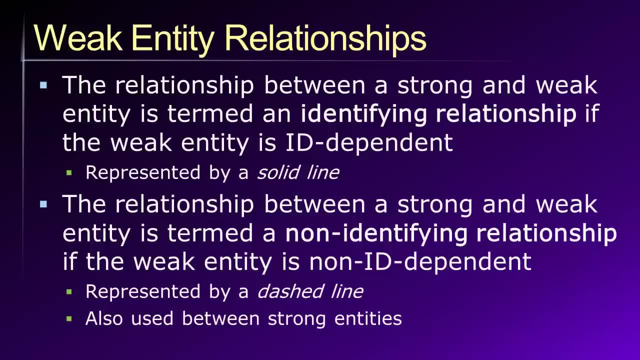 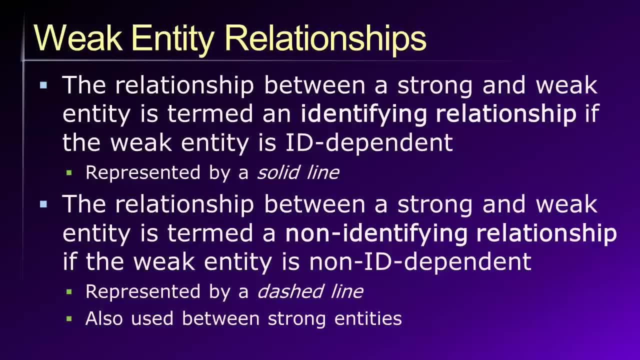 of a strong entity, then we call that a non-identifying relationship and we can say that the weak entity is non-ID dependent. In our entity relationship diagrams, in our Non-ID independent relationships, we are represented with a dashed relationship line and this dashed relationship line is also used to model. 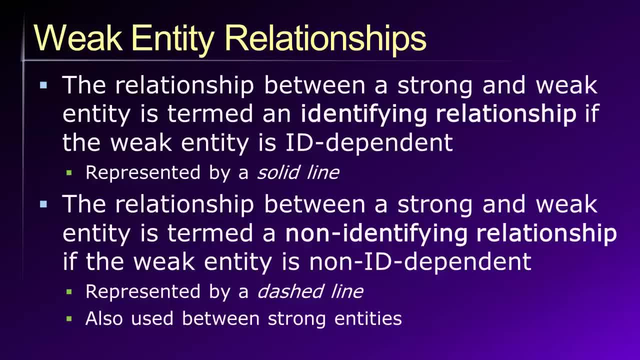 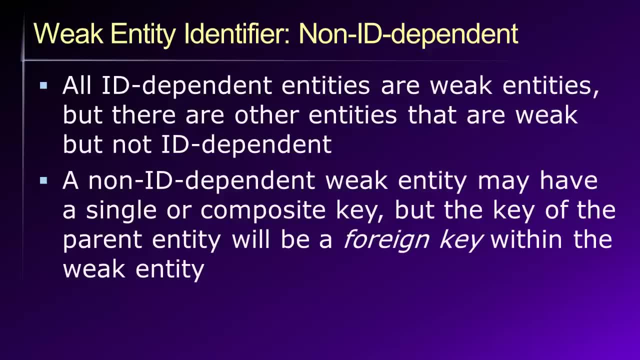 relationships between strong entities. If the relationship between a strong entity and a weak entity is non-identified, we can ID dependent relationship. then the primary key of the strong entity will appear as a foreign key within the weak entity. but it will not be a part of that. 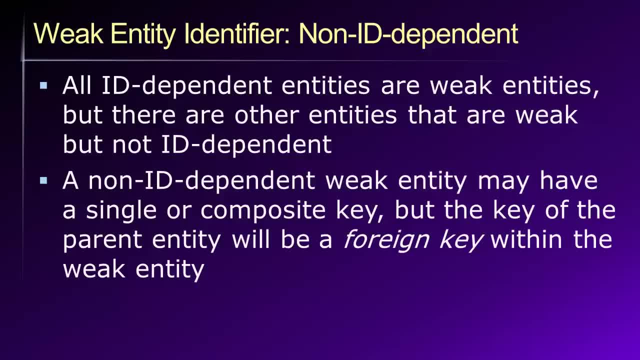 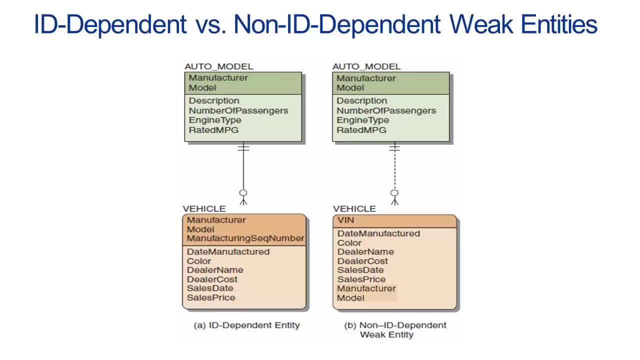 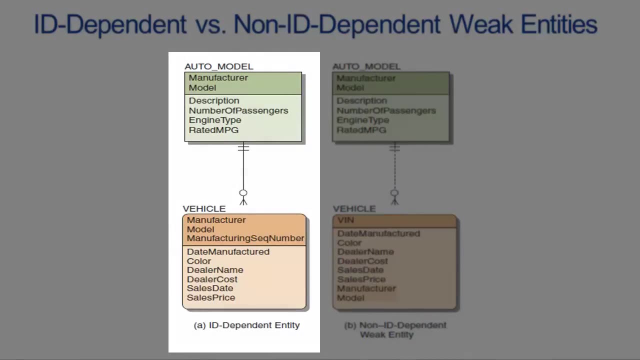 weak entity's primary key. Let's see some examples that will hopefully clarify the difference between ID dependent and non-ID dependent relationships. In our first example we see an ID dependent weak entity named Vehicle. We can tell that this is an ID dependent weak entity because part of its primary key is: 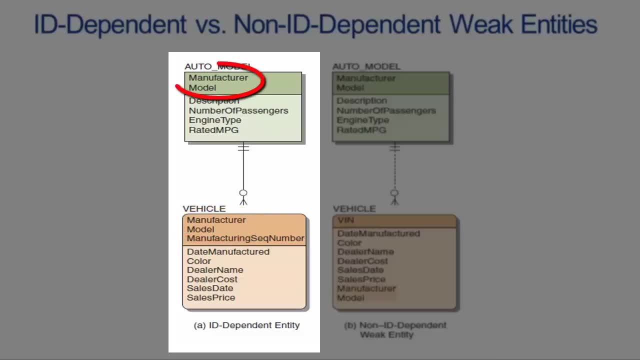 composed of the primary key from a strong entity. In this case, the strong entity is the auto model entity and its primary key is the combination of manufacturer and model, and in the vehicle entity we can see that manufacturer and model are part of the primary key. this is therefore an ID. 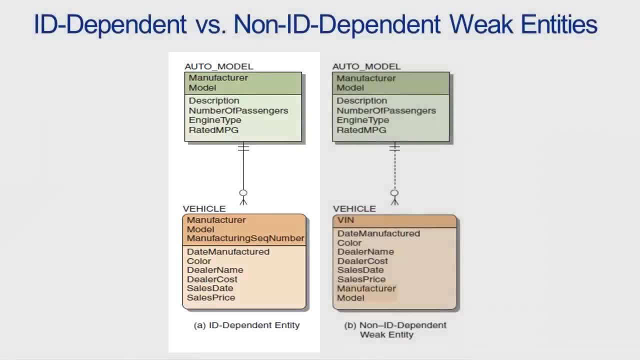 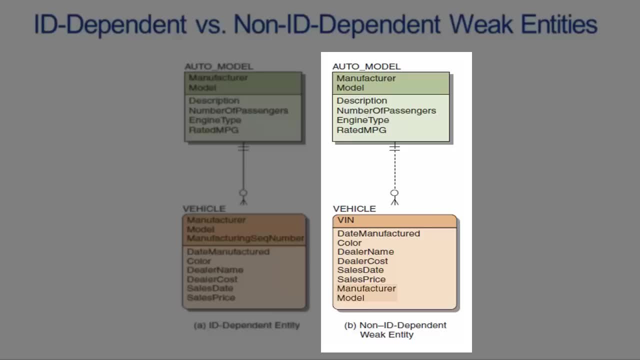 dependent weak entity. by contrast, we might use a different type of primary key for our vehicle entity, such as a VIN or a vehicle identification number, and in that case, the primary key of the strong entity- auto model- does not appear as part of the primary key of the weak entity vehicle. instead, the primary key 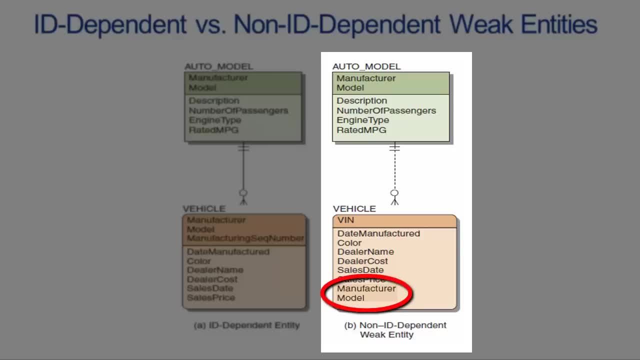 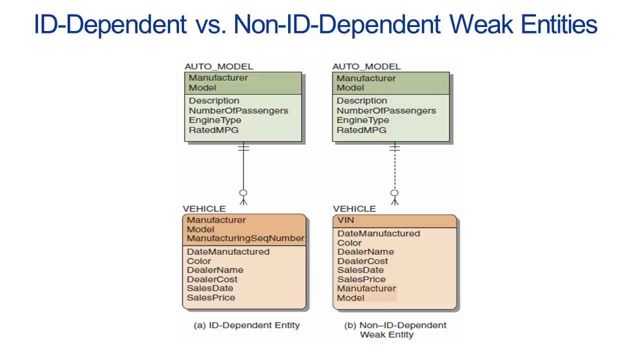 of auto model appears in the vehicle entity as a foreign key link back to the strong entity. in this case it would be a non ID dependent weak entity and again note that ID dependent relationships are shown with a solid line, while non ID dependent relationships are shown with a. 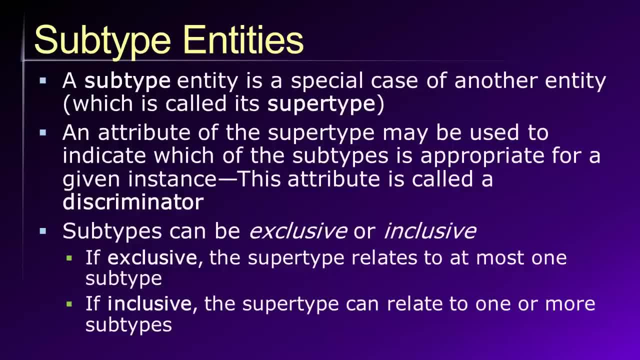 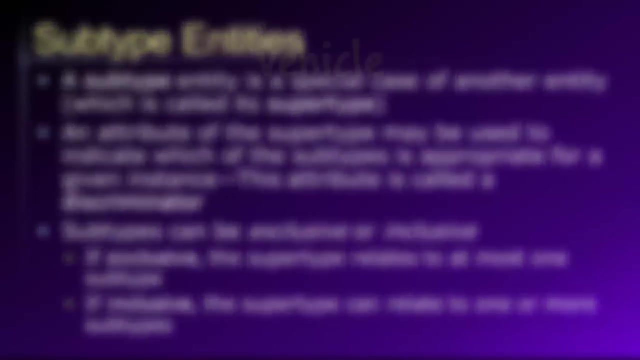 dashed line. next, I would like to talk about a different type of relationship between entities, which we can call a supertype- subtype relationship. in a supertype- subtype relationship, the subtype is a special case or a specific version of the supertype. as an intuitive example, Consider the generic concept of a vehicle. 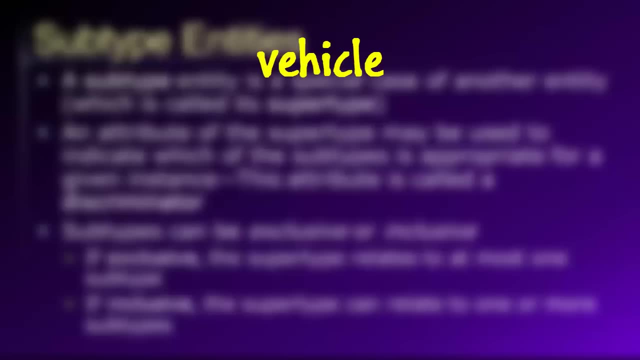 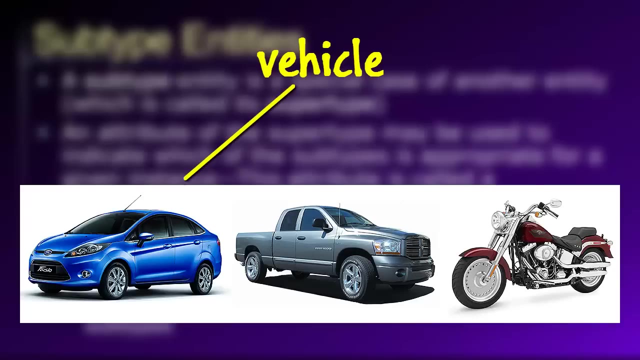 That might be a supertype, And then we might have specific subtypes of the vehicle class, such as a car or a truck or a motorcycle, where there may be unique attributes about a car or a truck or a motorcycle that we want to track, in addition to a set of attributes. 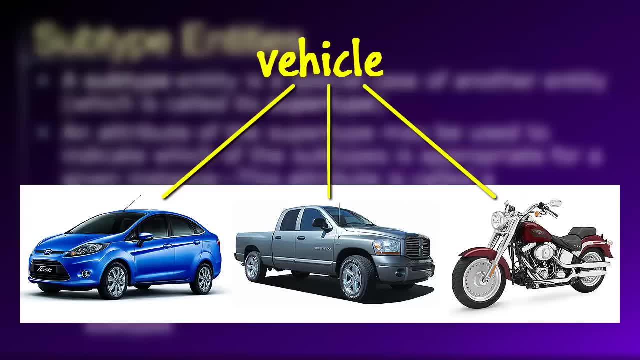 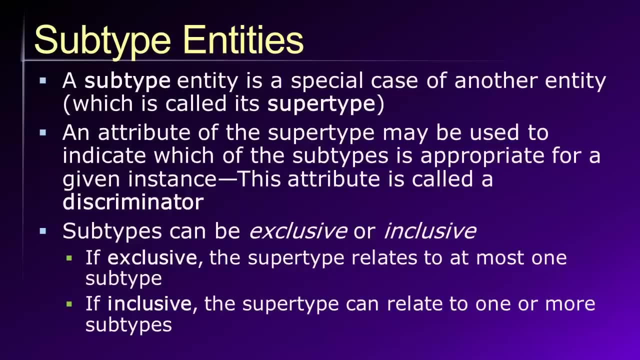 that we want to track for every vehicle, regardless of what specific type of vehicle it may be. This is an example of a supertype-subtype relationship. Broadly speaking, there are two different types of supertype-subtype relationships. The first is called an exclusive relationship. 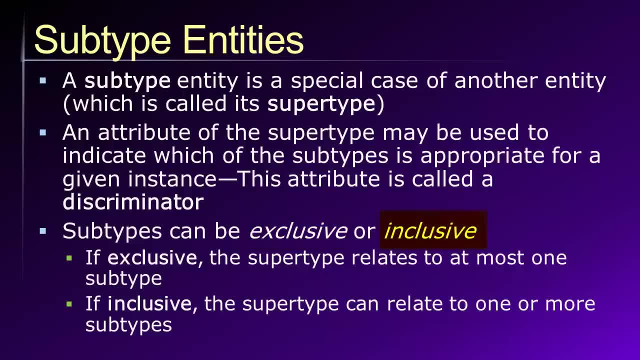 And the other Is called an inclusive relationship. If a supertype-subtype relationship is exclusive, what that means is that each instance of the supertype can be related to at most one of the subtypes. So a vehicle, for example, can be a car or a truck. 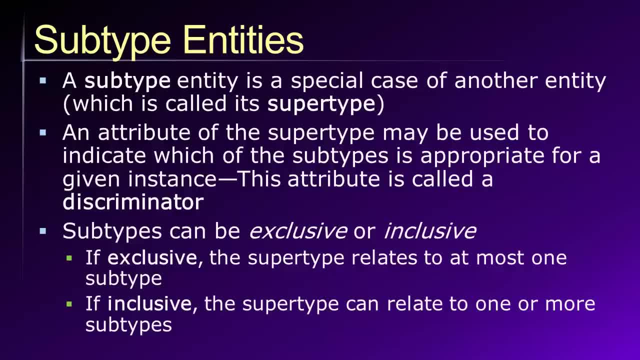 or a motorcycle, but it cannot simultaneously be a truck and a motorcycle. That would be an exclusive supertype-subtype relationship. By contrast, we might have inclusive supertype-subtype relationships, And in an inclusive supertype-subtype relationship the supertype can be related to one or more subtypes. 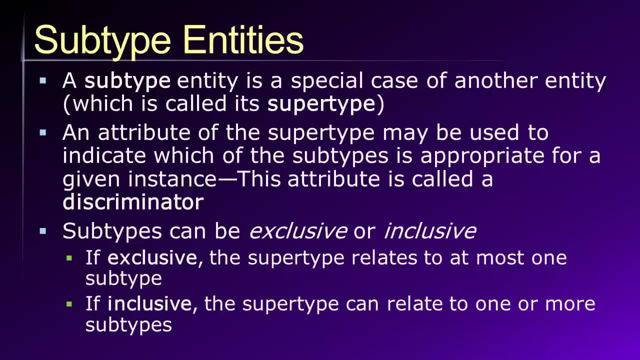 As an example, consider a university where we might have a supertype that we call person and we might have a subtype which we call student and another subtype which we call employee, In an inclusive supertype-subtype relationship, a given person at our university. 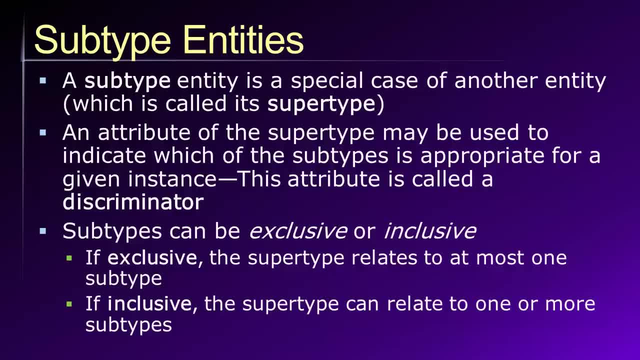 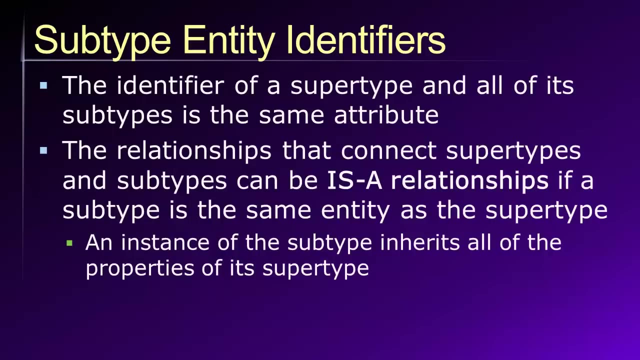 could simultaneously be a student and an employee of the university. Thus, when a supertype can be related to one or more subtypes, we call that an inclusive supertype-subtype relationship. In these supertype-subtype relationships, we will always connect supertypes to their subtypes. 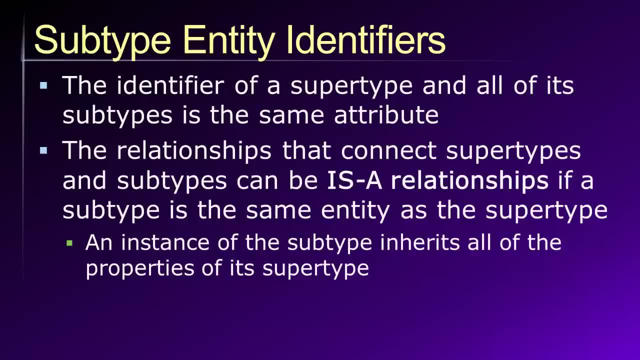 by using the same attribute. Recall that earlier we talked about the has-a relationships. So an employee has a locker or an employee has a parking space In supertype-subtype relationships if the subtype is a specific case of the supertype. 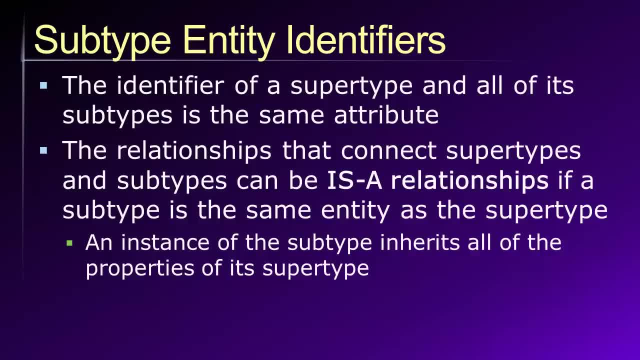 we say it is. So if the subtype is a specific case of the supertype, of the supertype, then we can call that an is-a relationship. Consider our previous vehicle example. A car is a vehicle, A truck is a vehicle. 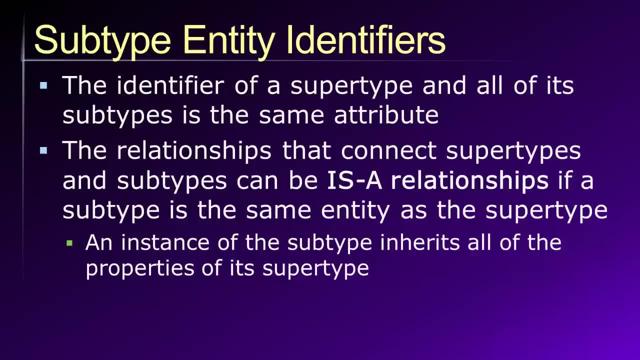 A motorcycle is a vehicle. Each of those three specific subtypes has individual characteristics which make it unique, but all three can be broadly classified as vehicles, types of vehicles. These are is-a relationships. Remember that in these types of relationships, in entity relationship, modeling, the subtype. 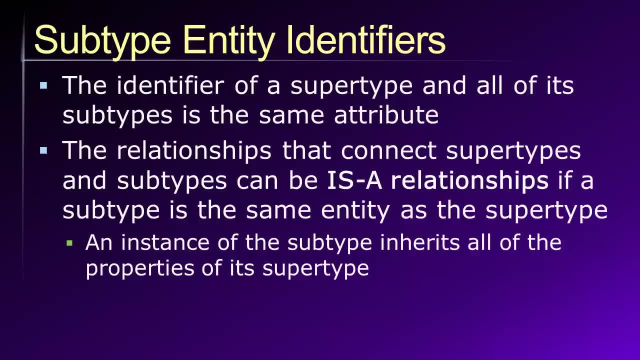 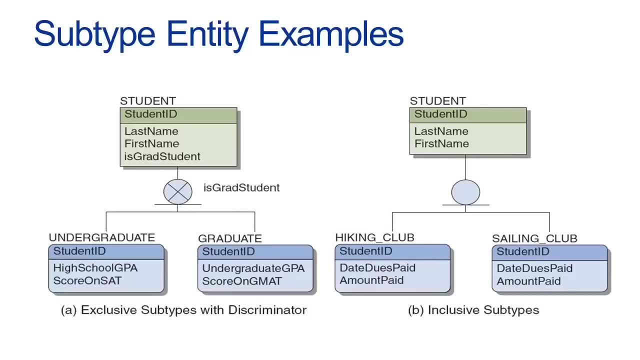 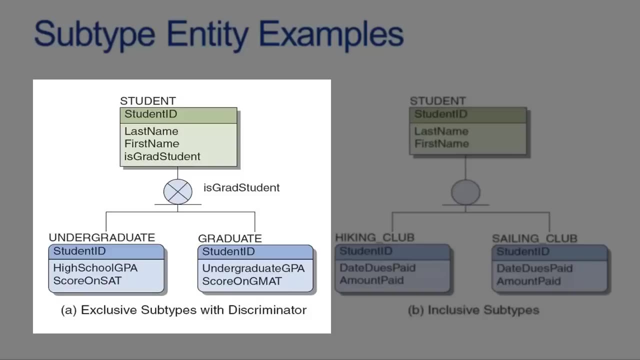 will inherit all of the attributes, all of the properties of its supertype. Let's see some graphical examples which will hopefully make these concepts easy to understand. In our first example we see a supertype-subtype relationship where the supertype is named student. 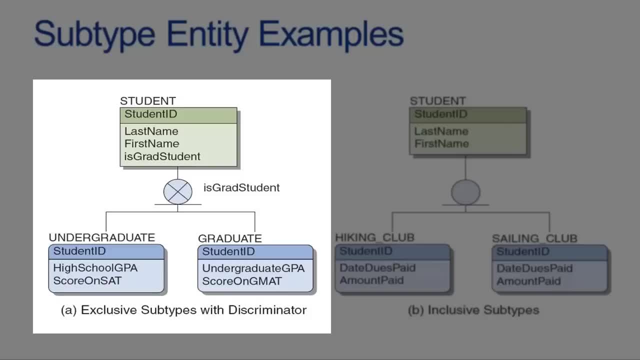 and we have two different subtypes, two different types of students. They are undergraduate students and graduate students. This is an example. This is an example of an exclusive supertype-subtype relationship, because a student is allowed to be an undergraduate student or a graduate student. 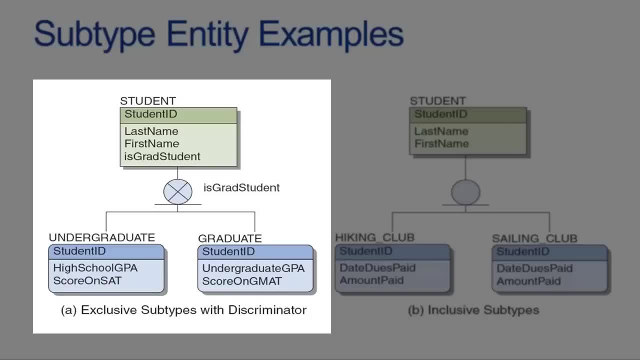 but cannot be both at the same time. Note here that we have an attribute in our supertype table named is-grad-student, for which we can imagine that values might be true or false, which tells us which of the relationship paths to follow in order. 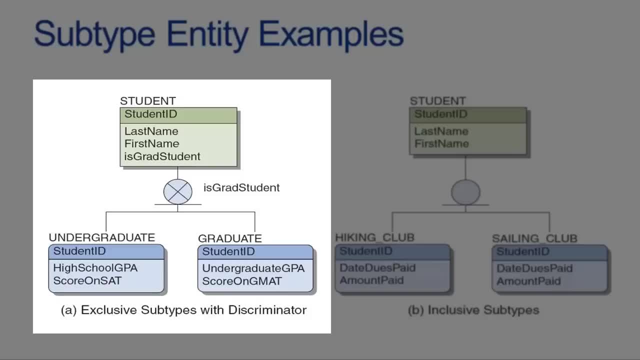 to get further information about this specific student. Also, note that each of the subtypes- undergraduate and graduate- contains attributes that apply only to that specific type of student. So a graduate student, for example, has an undergraduate GPA and a score on the GMAT exam, whereas undergraduate students. 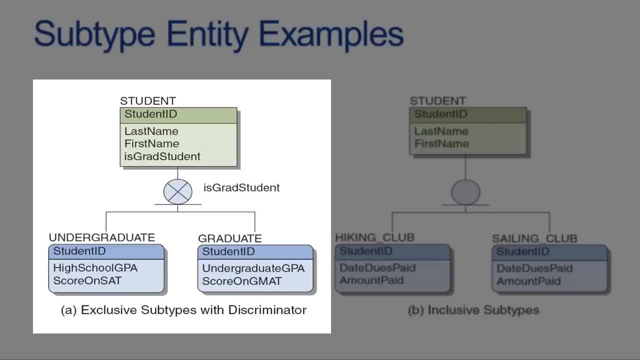 in this model do not have those attributes. Remember that when the subtype is a specific type of the supertype- in this case a graduate student- is a subtype. So if a student is a student, an undergraduate student is a student, then the subtype inherits all of the attributes. 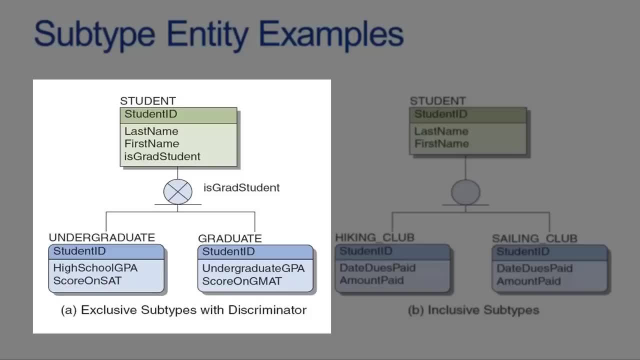 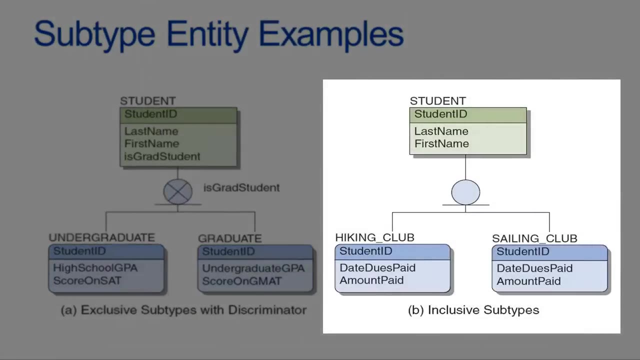 of the supertype. Also, note that we use student ID in order to link the supertype to the subtypes. In our second example we have an inclusive supertype-subtype relationship Where our supertype is a student and our subtypes. 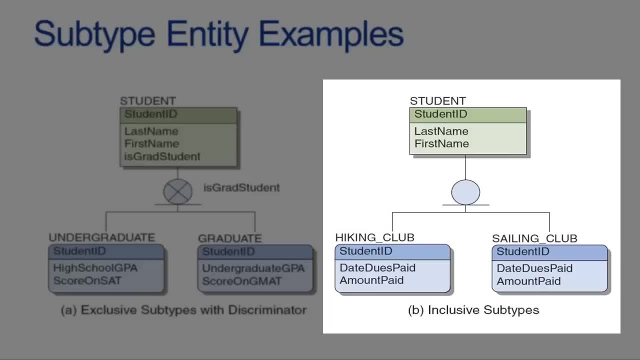 are various student clubs, So we may have a hiking club, a sailing club. Now, this is an inclusive supertype-subtype relationship, because each instance of the supertype- in this case each student- can potentially be related to more than one subtype. 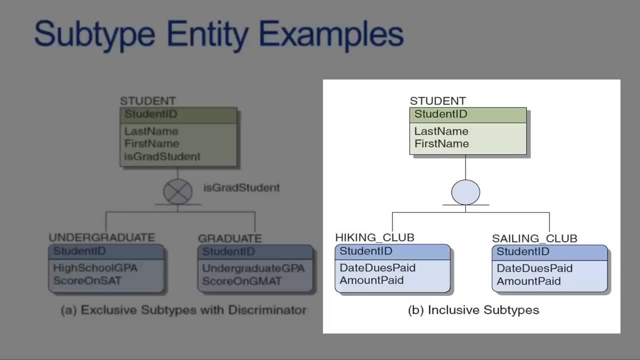 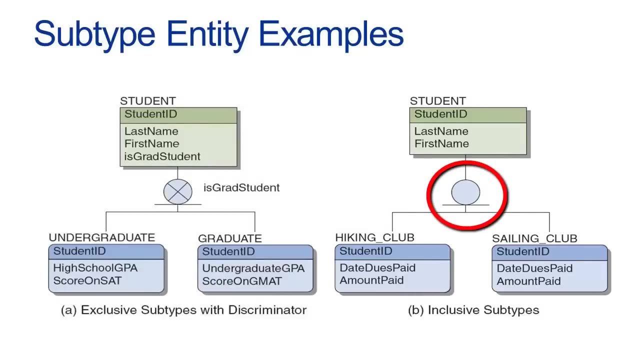 So a student Might be a member of the hiking club and the sailing club simultaneously. One last point to make on these supertype-subtype relationships. Note that we use this circular symbol with a line under it to indicate that a relationship is a supertype-subtype. 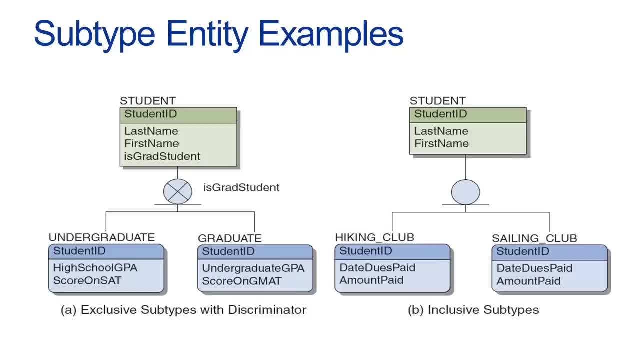 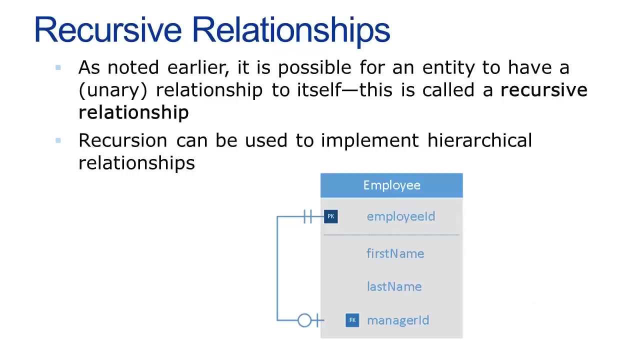 relationship. If an X symbol appears inside the circle, We know that is an exclusive supertype-subtype relationship, Whereas if no X appears inside the circle, we know that is an inclusive supertype-subtype relationship. As our last topic for this lecture, 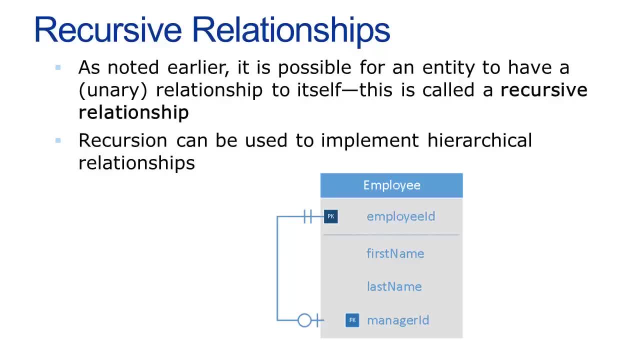 I would like to discuss recursive relationships. If you recall, earlier we said that it's possible for an entity To be related to itself in a unary relationship, And here we want to explore this concept in a little more detail. Consider this employee entity. 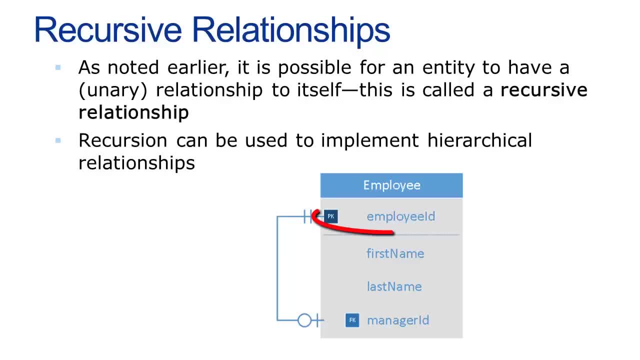 The primary key of the employee entity is employeeIfD And we have another attribute in this entity which is named managerIfD, And we see that there is a one-to-one relationship relationship between employee ID and manager ID In this example, the important thing to remember. 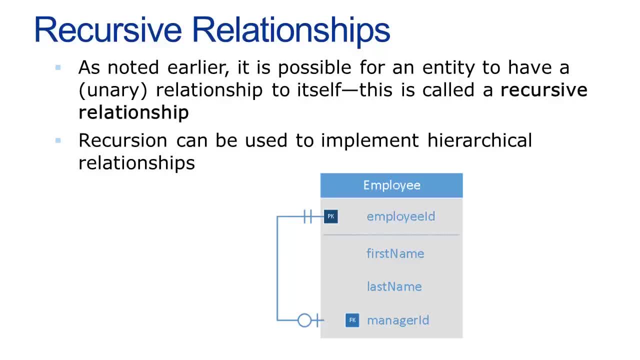 is that a manager ID is actually an employee ID. It's just being used with a different name here in order to allow us to map a specific type of relationship between employees. These types of recursive relationships can be very useful for tracking things like customer referrals. 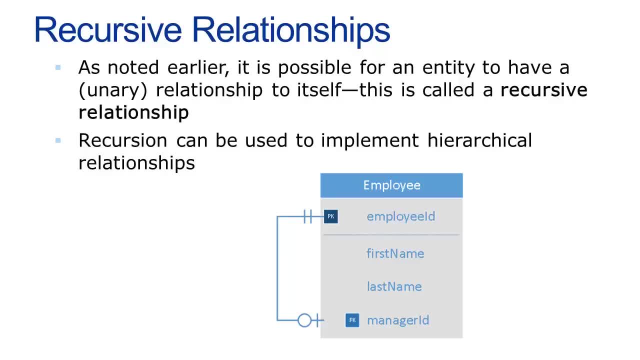 For example, imagine that we run a dentist's office. Each customer that we have- each patient, if you will- might have been referred to us by another patient And we might want to know: well, what do we want to keep track of that information? 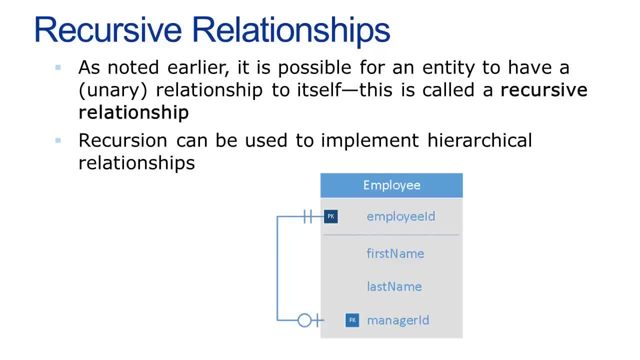 We can track that information in our customer table or our patient table by using one of these recursive relationships. Another great use for these recursive relationships is to implement hierarchies, And that is what can be accomplished using the sort of design that we see here. 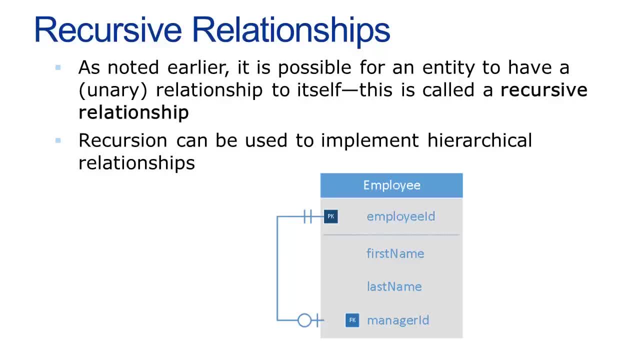 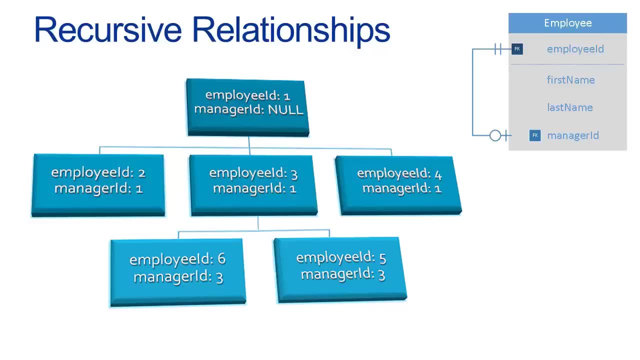 with our employee entity. Let's see how this works in more detail. Each of the rectangles that we see here represents a record or a row in our employee table. At the top of our hierarchy we have employee ID number one, And for this employee ID the value of manager ID is null. 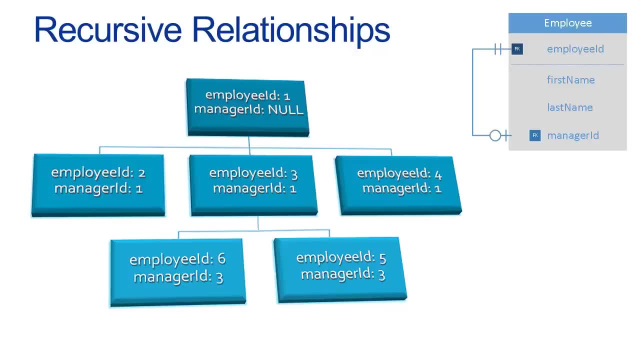 And what this tells us is that employee ID number one has no manager. So we might imagine that employee ID number one is the CEO of the company, for example. Moving down to the next layer in the hierarchy, we have employees two, three and four. 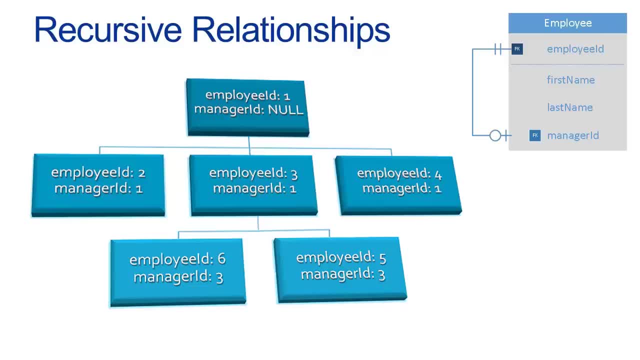 And for each of these employees, we see that their manager ID is one. So this tells us that employees two, three and four are the managers of the company And for each of these employees, we see that their manager ID is one. 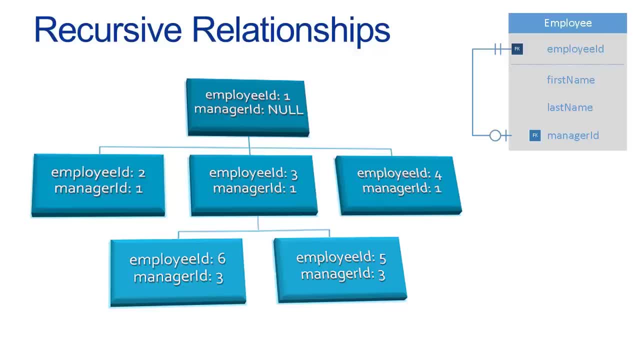 So this tells us that employees two, three and four report to employee number one, Or another way of saying that is: employee number one is the manager or the boss of employees two, three and four. Further down in the hierarchy we have employees five and six. 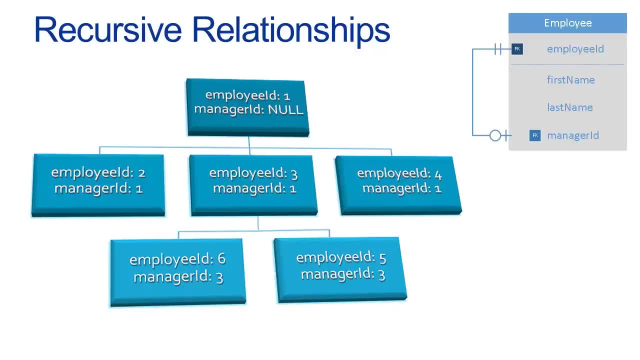 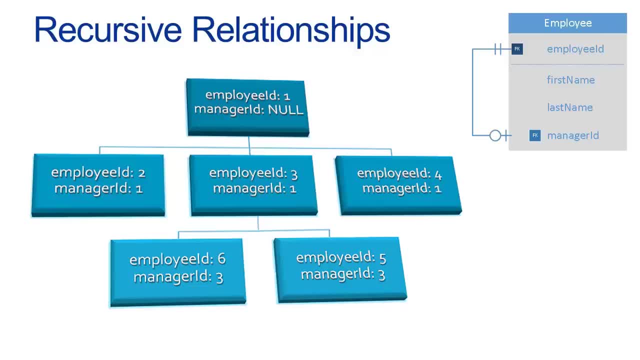 And employees five and six have a manager ID of three And employees five and six have a manager ID of three. Employees five and six work for employee three, who in turn works for employee one. By implementing this sort of recursive relationship, I hope you can understand how we could easily. 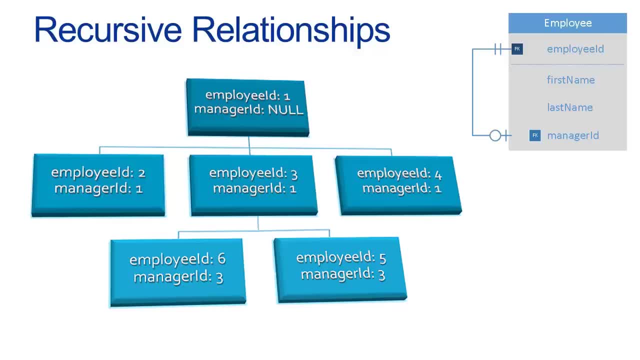 track the hierarchical relationships among employees and managers for an organization that has as many levels of management as we want and as many employees as we want. We could use this approach to track employee-manager relationships for a small company containing as few as five or six employees, like the example we see here. 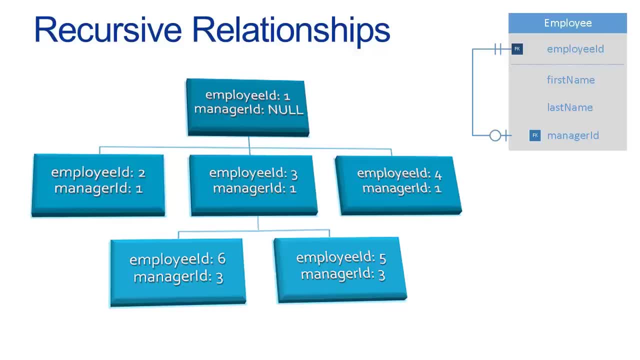 But we could use exactly the same approach to track all of the employee and employee-manager relationships for a massive company, For example, a automobile manufacturer that might have nine or 10 levels of management and tens of thousands of employees. The point to take away from this example. 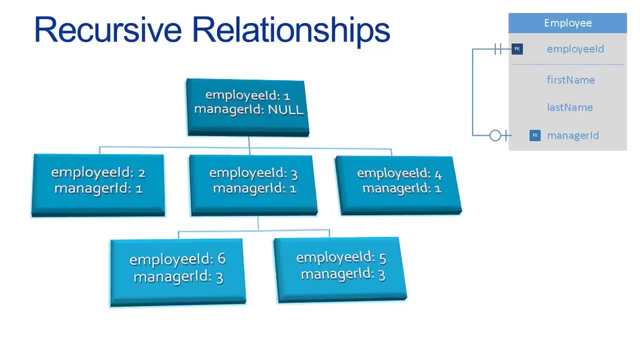 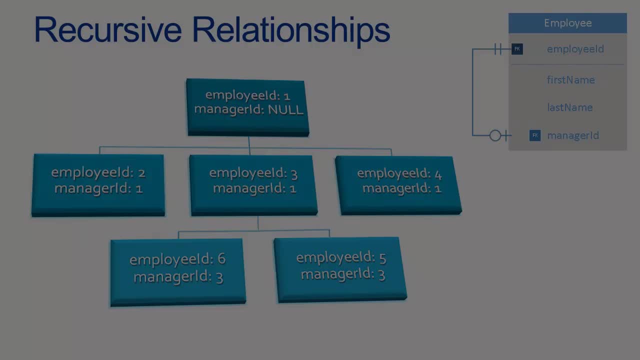 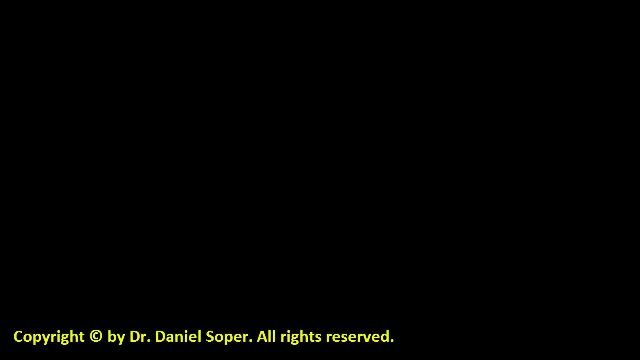 is that we can implement a hierarchy of any arbitrary level of complexity using just this simple data modeling approach. Well, my friends, thus ends our brief exploration of data modeling and the entity relationship model. I hope you learned something interesting. Until next time, have a great day.